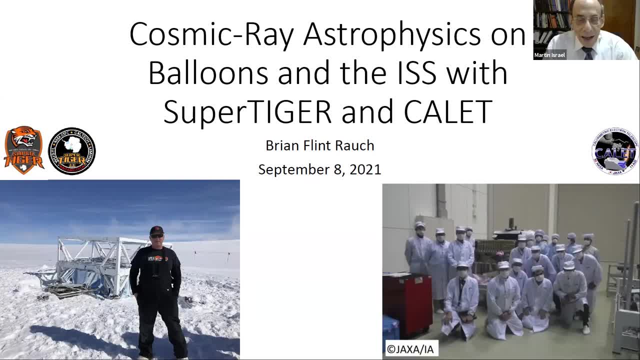 and he was very involved from the beginning of his undergraduate days. He was very involved from the beginning. This same program was the meat for his PhD when he returned and he has had a key role in the SuperTiger development out of Tiger since then. In Calette, the other major experiment, he'll 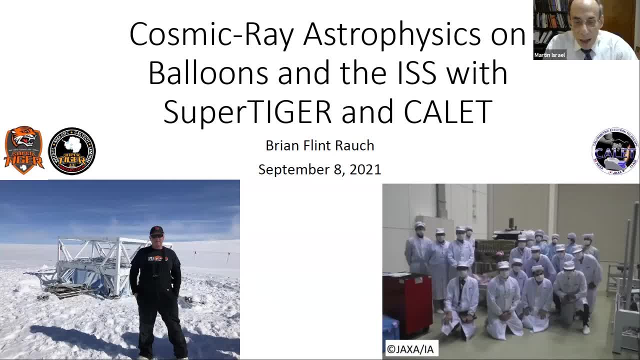 be talking about. he's had a key role from the beginning of WashU's involvement and Bob had been the PI, But a couple years before his retirement a few years ago, the PI ships of both of these things and another experiment that's not on the docket today has been in Brian's very capable hands. 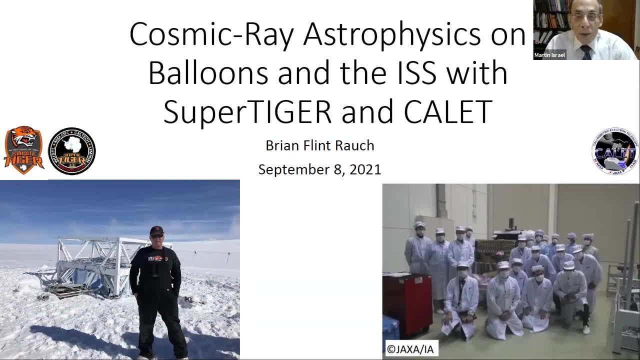 So it's really a pleasure. It's a pleasure to hear from Brian about what's been going on with SuperTiger and Calette. Brian, welcome or re-welcome, All right. well, thank you. I haven't been introduced since I defended. 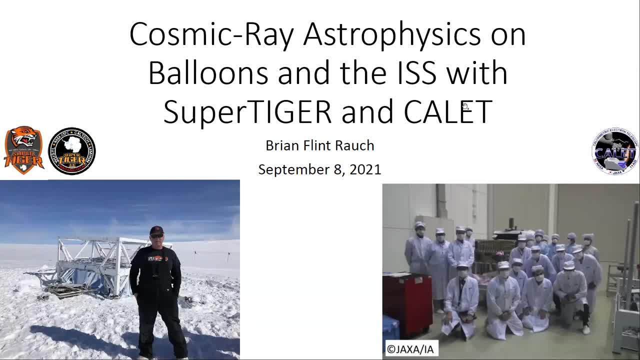 And I haven't lectured here since I did a grad student seminar a long time ago. All right, so, as has already been said, cosmic ray, astrophysics on balloons and the ISS with SuperTiger and Calette. So we have pictures from each. 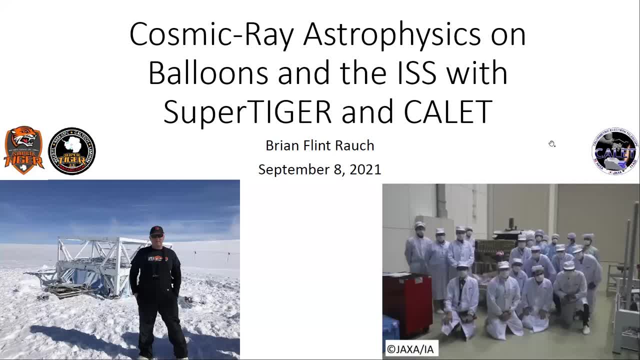 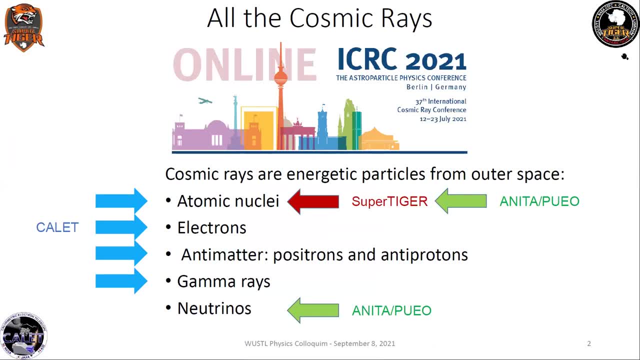 Hopefully this didn't get clicked on there. We'll just click on it. Oops, getting ahead of myself. At least I don't have any videos this time, So you know. one question is: oh, can I hide this? Does anybody make this not show up? 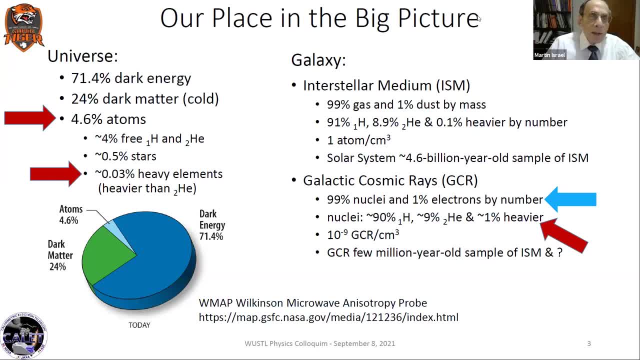 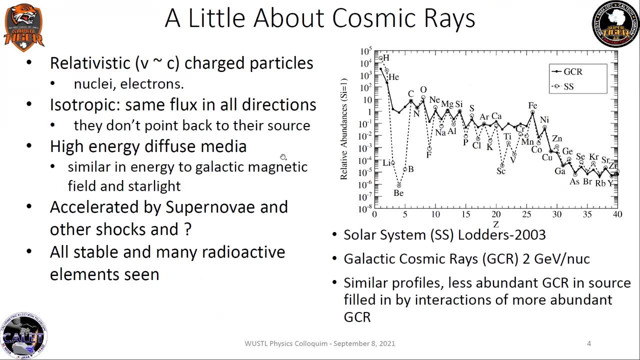 Everything's fine. now I'm just seeing what I think you want us to see. Oh, okay, that's fine. Sorry, it shows up on the screen here. It might just be for you. yeah, Well, it's also showing up on that screen. 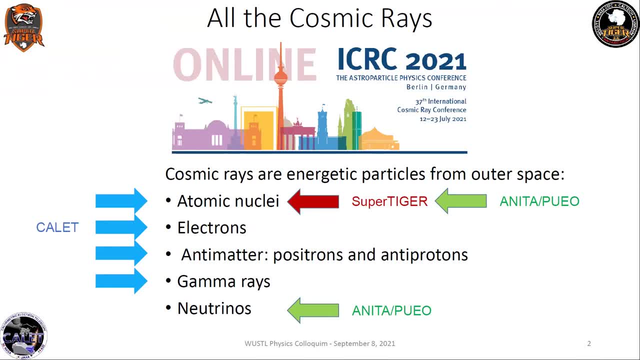 Yeah, so anyway, And moving on, This is probably about as out of the way as it's going to get. Yeah, All right. so all of the cosmic rays. Someone wanted to know what all of them were And just having recently done the International Cosmic Ray Conference in Berlin, 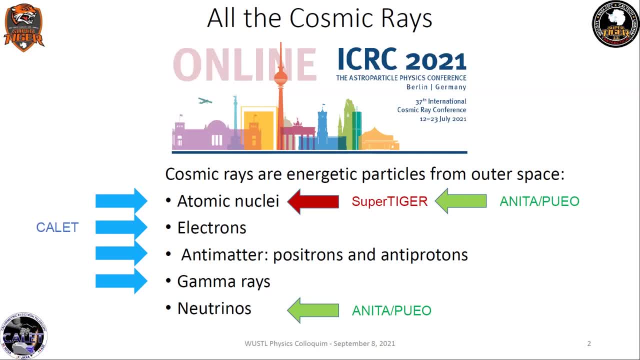 remotely, which was no fun. I don't recommend international conferences remotely personally And what I recall. of course, the cosmic rays are energetic particles from outer space. They come from outside the solar system and also the sun in some cases, And they include atomic nuclei electrons with antimatter, mostly positrons and antiprotons. 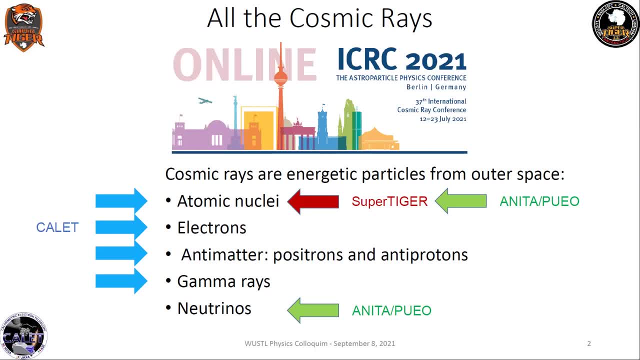 so that people search for other things. They include gamma rays and they include neutrinos, And when I was going to do this PowerPoint, I'd have these arrows popping up and saying: they're all like an atomic sequence, but they're all up at once. 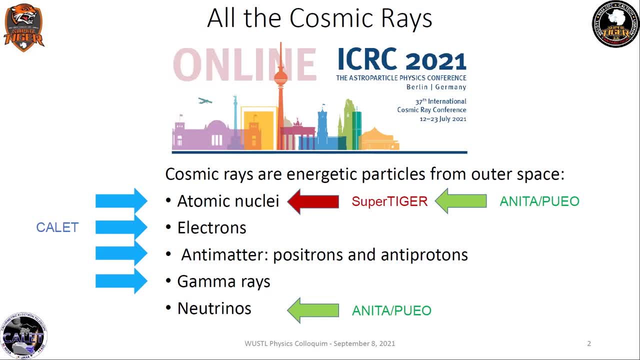 CALLETTE on the space station covers just about everything to some degree except neutrinos. SuperTiger is entirely focused on atomic nuclei and the heavier ones of those, And I'd also mention Anita Puello briefly, because that's another experiment we work on here. 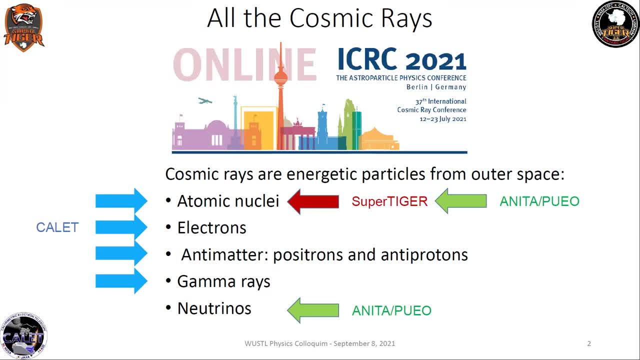 I've worked on and took over from Bob, And it is designed to measure the highest energy, neutrinos, but it also measures the highest energy, ultra-high energy, cosmic rays, degrees with atomic nuclei, Because I touched that, All right, great Again. this is all. 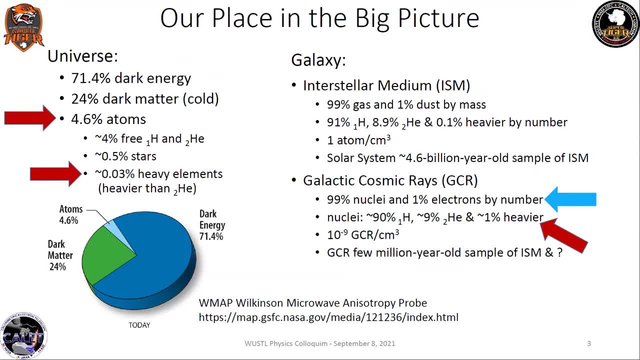 going to be so fancy. Now we're PDF, So what's the place of the big picture for this right? So the universe is mostly dark energy: over 70% dark energy, almost a quarter of dark matter, and then just a small less than 5% of atoms. So, of course, not being the kind 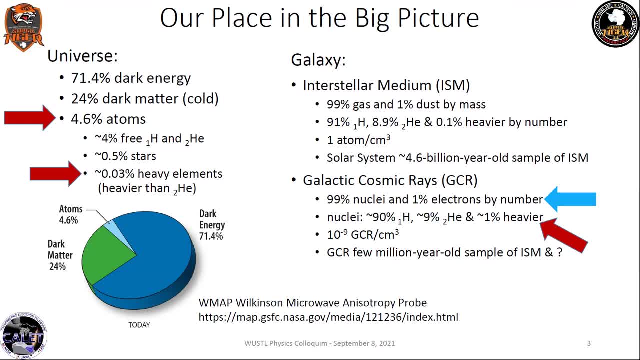 of person to go after a Nobel Prize. I'm going to focus on the more mundane atoms, And of those, about 4% of that is hydrogen helium, so it's mostly just pure hydrogen helium. only 0.5% stars and a tiny 0.03% is heavy elements, And by that you just mean 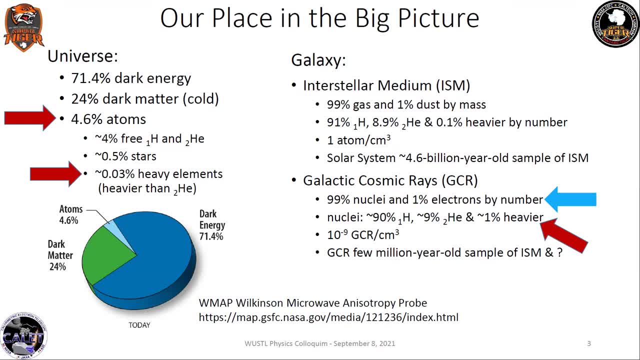 metals. If you're talking like an astronomer, it's heavier than helium. So that's that fraction. And then we switch from the big picture view of the universe over to the galactic view And we have two samples of interstellar medium to consider. 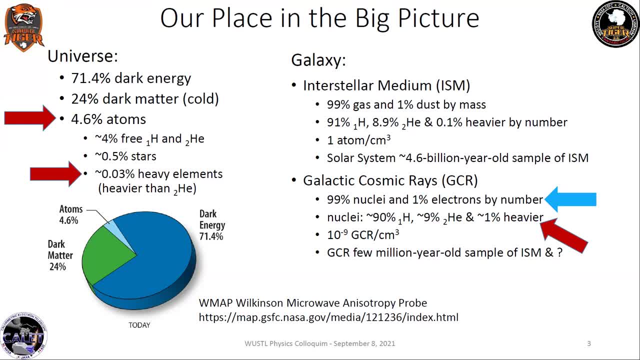 In the galaxy. one is the solar system. It's about a 5 billion year old sample, 4.6 billion year old sample of the galactic material And it has most of its gas, about a percent of its dust by mass, and 91% hydrogen, almost 9% helium and just a tiny 0.1% everything. 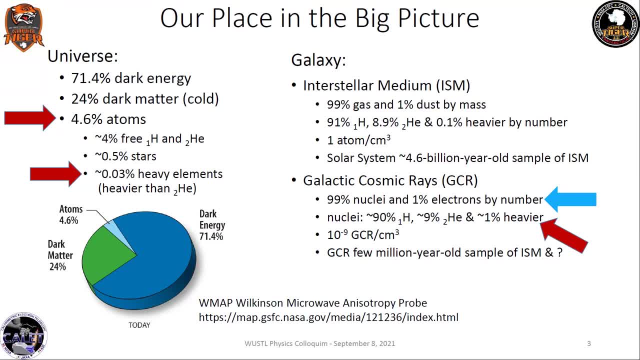 heavy. Then there's the galactic cosmic rays. This is a much fresher source of galactic material. It's a few million years old And it's a sample of some isotope- Same ISM, we think, but we're not exactly sure what else is mixed in- And it's much 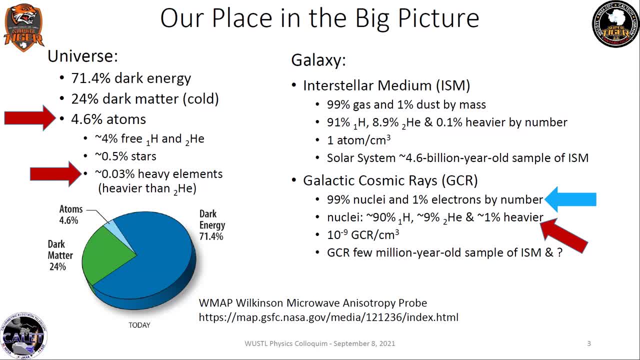 thinner. So the ISM in general is an atom per cubic centimeter, but the cosmic rays are 10 to the minus 9 per cubic centimeter, So it's a thin rain, as someone in this group once upon a time called it. The fractionation: it's 99% nuclei and 1% electrons, And that's 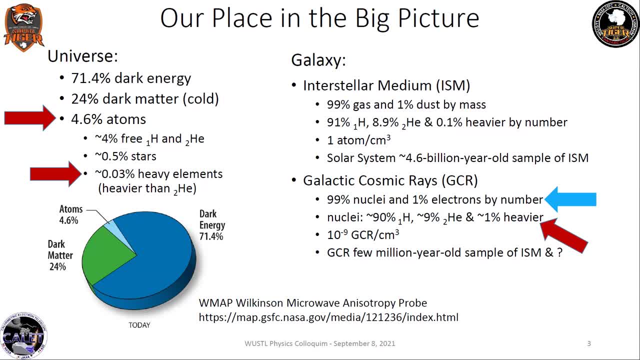 significant because the Calumetric Electron Telescope is designed to measure electrons. specifically, It measures base energy electrons, but it also measures nuclei. And then the nuclei are 90% hydrogen, 9% helium and 1% heavier things, And it's the heavier things that we're. 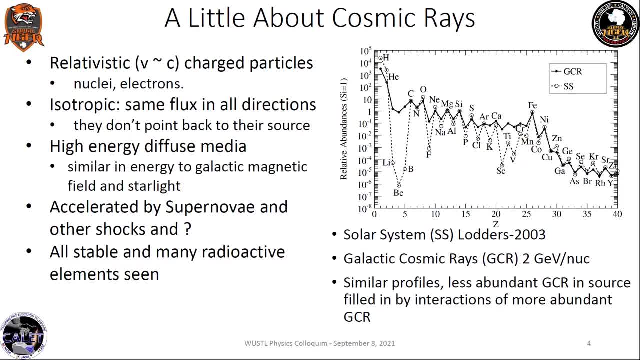 most interested in here at WashU. So a little bit about cosmic rays. They're relativistic charged particles, at least the ones I'm going to be talking about in this talk- nuclei and electrons. So we're going to neglect all the other ones we already mentioned, except in passing through Cal-Lit. 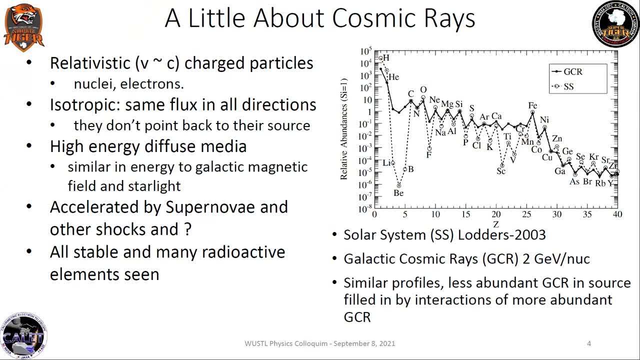 Cosmic rays are isotropic, which is to say that they come The same flux from all directions. They don't point back to the source, And that's because charged particles are deflected by magnetic fields. And even though the galactic magnetic fields are weak, they're very large scale And by the time cosmic rays get any real distance, 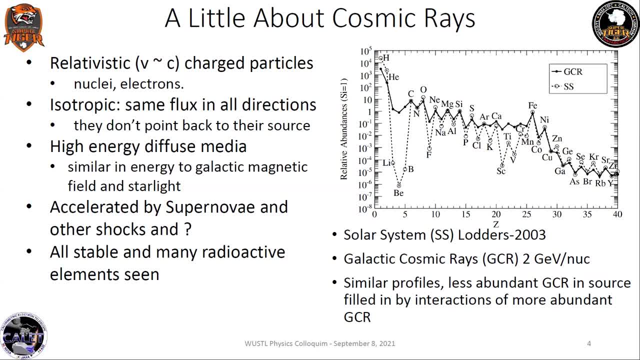 from the source. they've been randomized in direction. They're very high energy. Of course they're naturally speaking, since we're talking about relativistic. They're accelerated by supernova, shocks and probably other sources besides. And when we look at the cosmic rays, 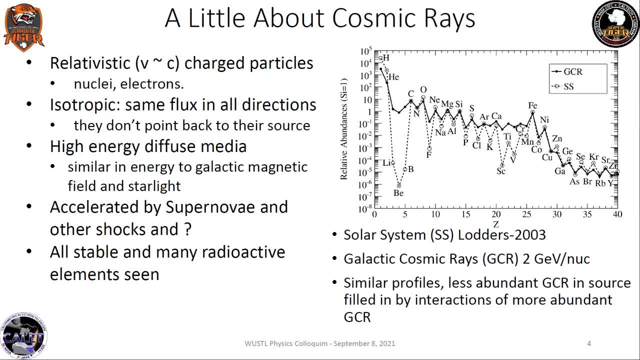 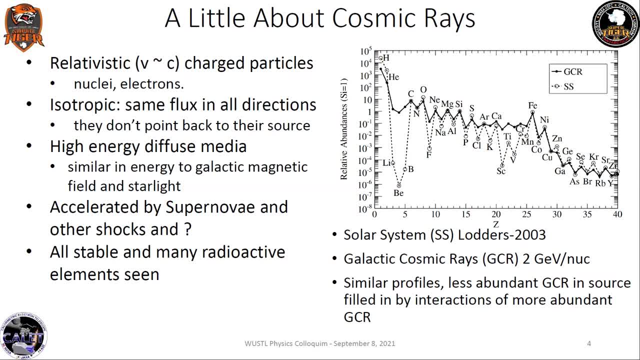 have observed both stable and radioactive elements there as well. So when we talk about cosmic rays, it's natural to compare them to the solar system, And when we do that, we use solar system abundance from Katerina Laders- And this plot is using 2003,, but she's 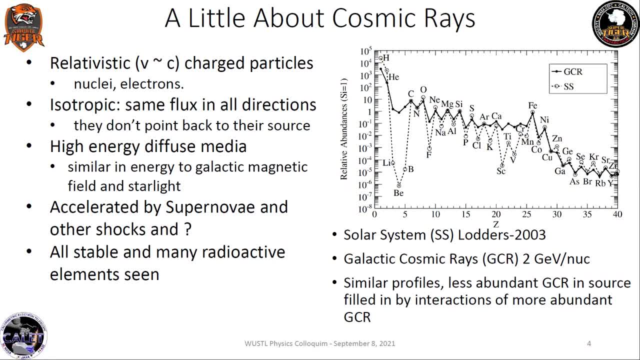 constantly producing Improved and updated abundances and we just haven't necessarily get around to using them. The galactic cosmic rays plotted are for 2 GeV per nucleon, And so I'm comparing from hydrogen up to zirconium, which is charge 40. And you see that there's a lot of similarity. 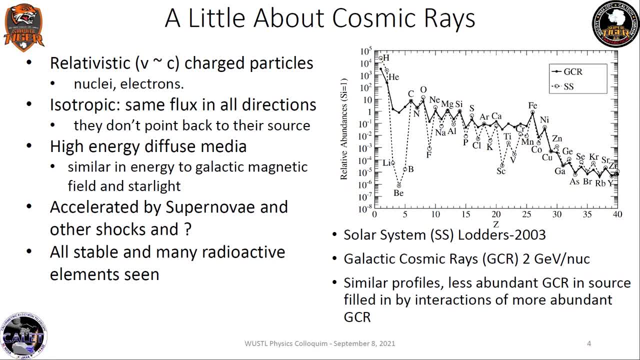 between these trends. And also, I should point out that you normalize a silicon equals one, And so there's a lot of similarity, but there's some real differences. And solar system, you know, is, There are a lot of places where they're. 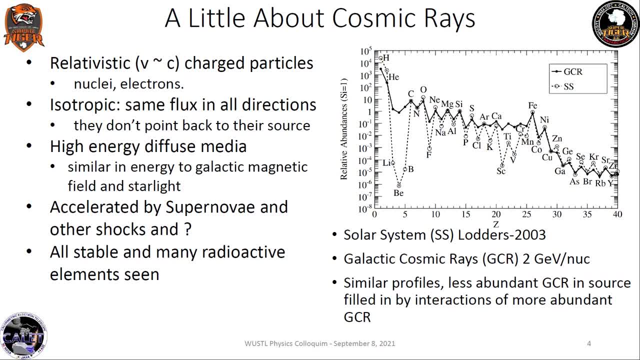 There are major valleys where the solar system is compared to the cosmic rays And in some instances, a lot of instances. that's because the cosmic rays interact on the way here. They travel through, you know, a few grams per cubic, Few grams per centimeter squared of density of material on the way here. But that's enough. 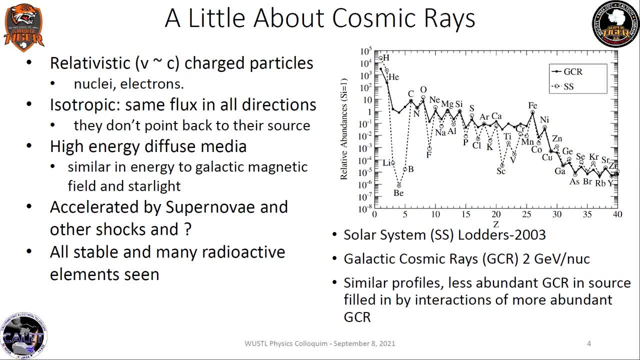 to induce a lot of fragmentation, And so the lithium, beryllium, boron at the bottom periodic cable there are particularly sensitive, And this is actually a major source of those elements is how they're synthesized from, But otherwise they're broadly similar, And it's where we look at the differences we can. 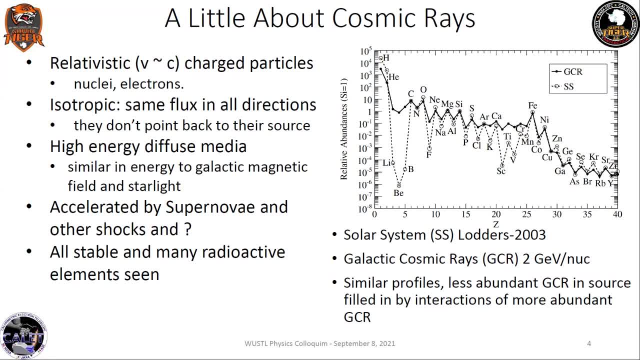 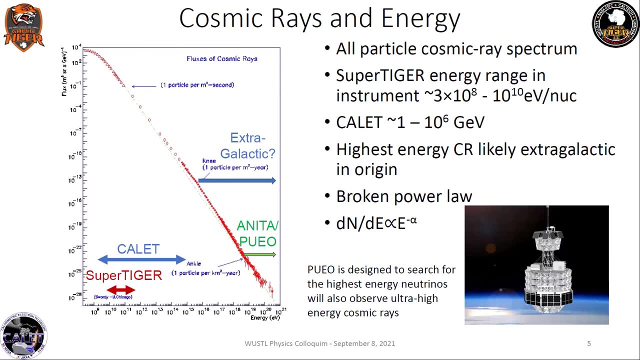 see above the, Above, the iron peak, which is the end of fusion. that helps point to source information. Okay, So cosmic rays and energy. The plot here on the left is the old particle energy spectrum. So it's everything, but that's dominated obviously by protons, since that's 90% helium. 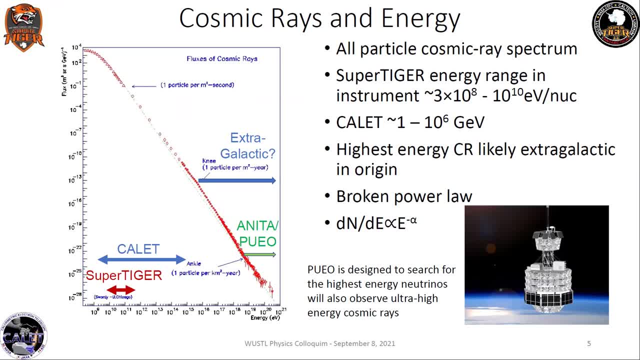 but it's another 90%. You see, you span many orders of magnitude and energy and flux And I plotted where SuperTiger and CalET fall on the energy scales And you can see SuperTiger is much lower- It's a much smaller range and lower total reach- than CalET. CalET is specifically designed. 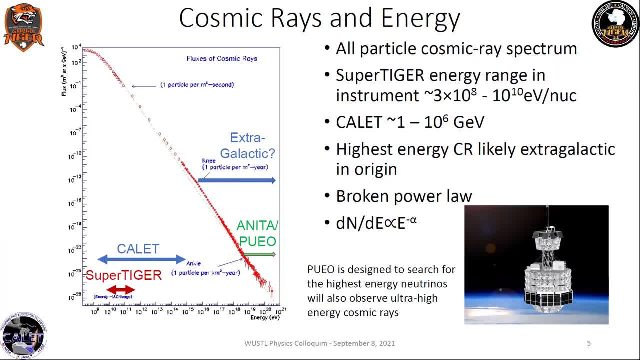 having been designed to measure and make direct measurement of the highest energy electrons as a deep calorimeter, that enables it to make those measurements. You see, there's a feature called the knee, above which people believe that the sources are extra galactic and not as well understood. We don't know exactly what it is, although there are theories involving 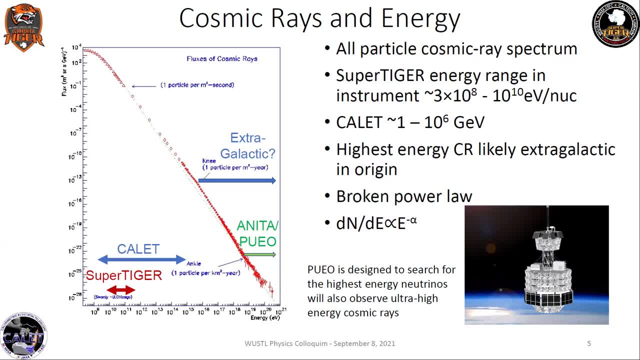 active galactic nuclei And the high end of the scale, various in the scale, like the highest energy particles, will have the momentum of a majorly fastball and they smack into your satmasphere, Which are, But they're obviously very, very rare And the problem, You can see that the particles 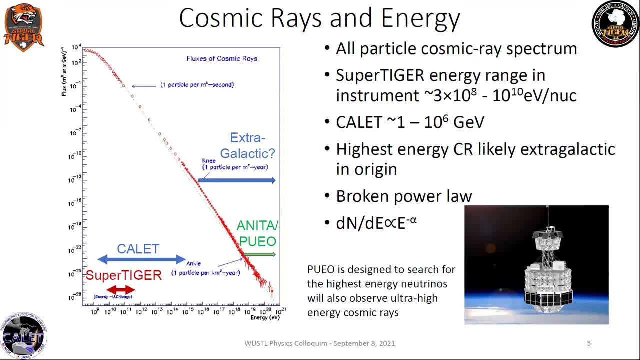 per meter per second and. And the problem. You can see that the particles per meter per second and. And the problem. You can see that the particles per meter per second and Metersquared year and Kilometersquared year Pointed out there. 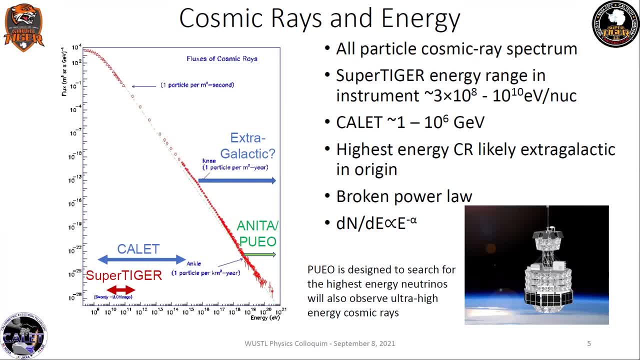 So in order to observe these rare high-energy particles, you need either and or both: a large detector or a whole lot of time, and usually both. And when you're looking at the highest energy ones to observe them, people will look at the atmosphere, large sections of the atmosphere. 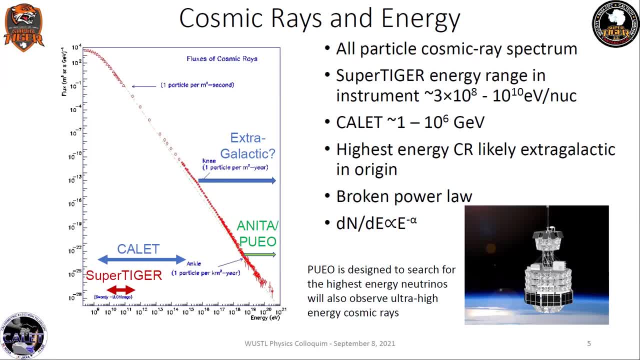 but look up at the sky, Or in the instance of Um, But They'll look down Or look across from a Uh, stratosphere point of view. So SuperTiger's energy range 300 MeV per nucleon to 10 GeV. 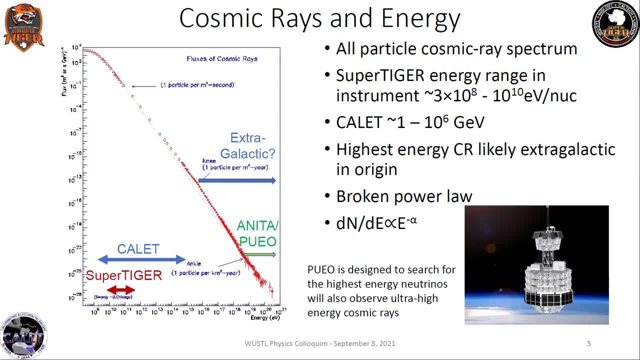 per nucleon cal lights 1 to 10 to the 6 GeV total energy. So when you speak of per nucleon, you're saying per, you're getting- yeah, it's kinetic energy- versus the total energy. The calorimeter has the total energy, so that's why we speak of it in the different 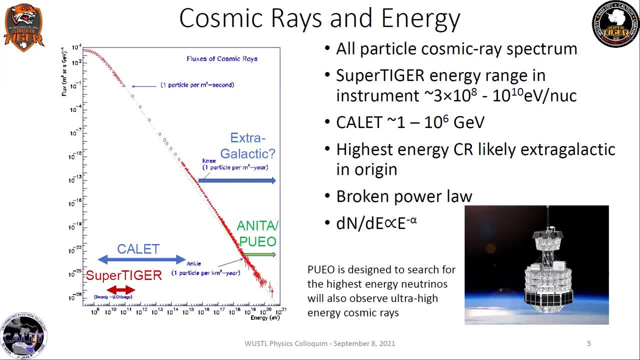 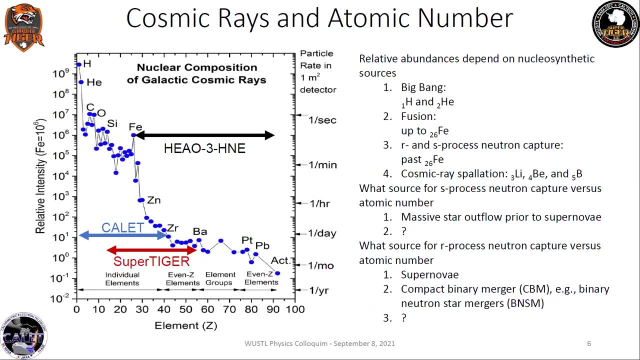 terms there: Ice energy, as I already said, they're extra galactic and we'd rather talk about the power law. All right, so calcium is an atomic number. So, since we're focusing on nuclei, again, hydrogen and helium are dominant, but you see also that this the 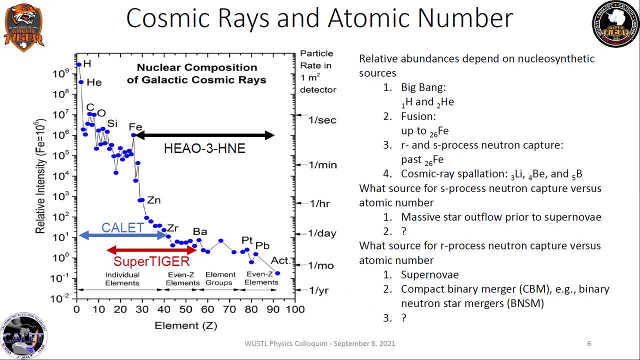 relative abundances of these elements fall off very steeply, especially below hydrogen and helium, but then again at iron, And the ultra-heavy calcium is above iron, particularly zinc and up. That's what we are focusing on. We're focused on measuring the SuperTiger, but we also can make a significant measurement. 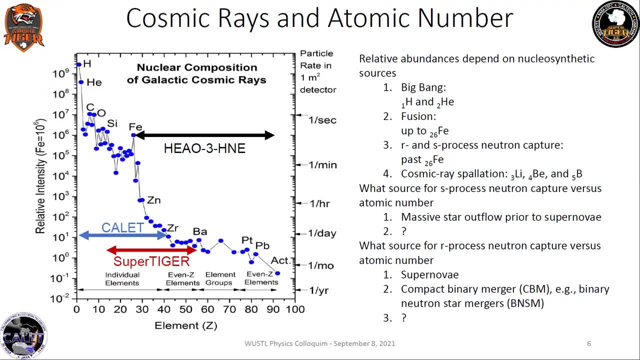 with cal light through zirconium And on the left, on the right margin, you can see the particle rate for just a meter squared detector as a function of, as a function of atomic number or element, And you can see that they get very quickly, get very rare as you get. 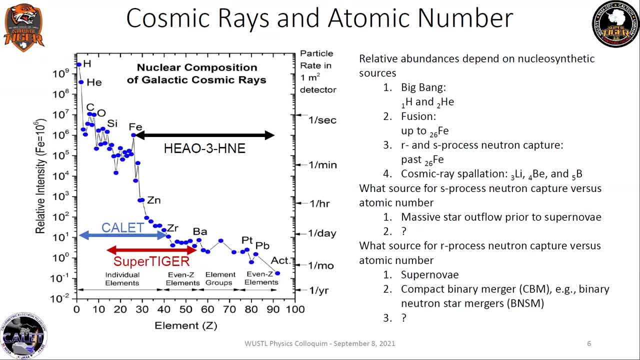 into the UH range And so again there's a real premium for both size and or duration of collection. And I note also HEO3-HNE, the heavy nuclear explorer. This was an instrument of Bob and Marty- Bob Benz and Marty Israel were leaders on- And it made the best measurements to date. 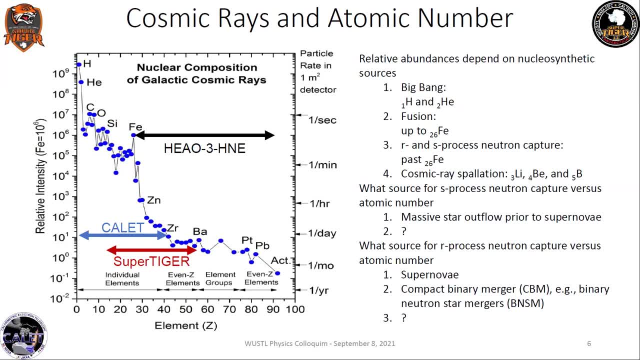 for elements toward the end of the periodic table. Its sentiments are planted, at least a part of this range, by recent SuperTiger measurements that I could be showing you. So the relative abundances, you know what's made where right Hydrogen and helium come. 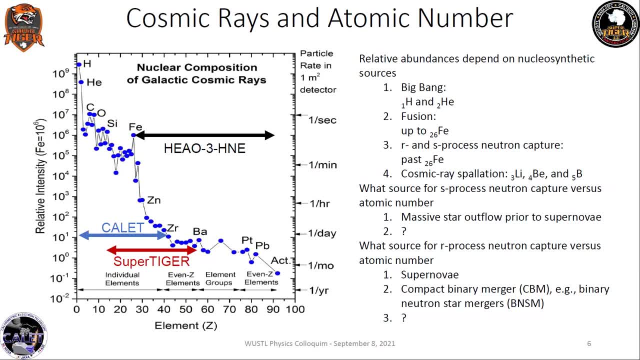 out of the Big Bang And then up to iron- it's mostly zinc- and up to helium, And that's what we're focusing on here. So if we go iron it's, it's a fusion, for the most part, with some cosmic. 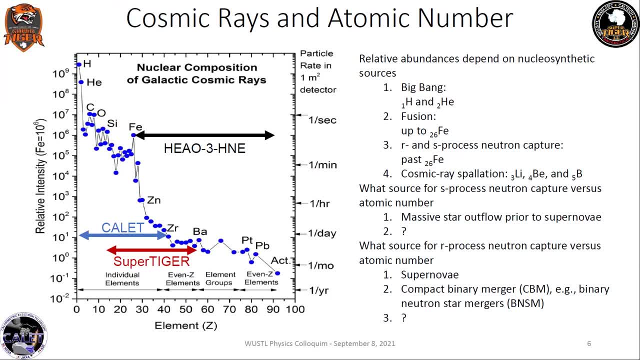 ray spallation production And then beyond iron- though it's a rapid or slow process- neutron capture, And I didn't mention spallation's nice. So S-process happens slowly, right By definition, And it happens over the lives of stars, while 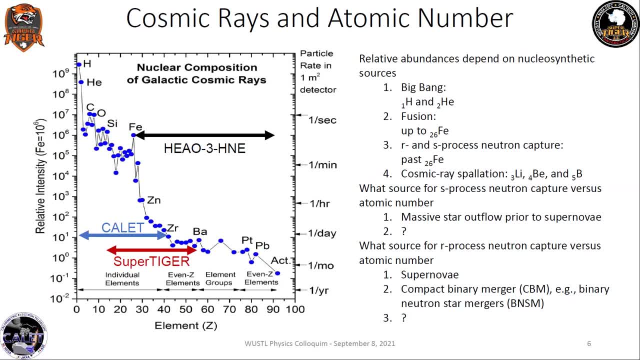 they're doing. while they're burning and fusion's ongoing And heavier nuclei will pick up new that get produced just in decays and other reactions within the stars and very slowly build up the nucleus, with plenty of time to decay back to stability along the way. 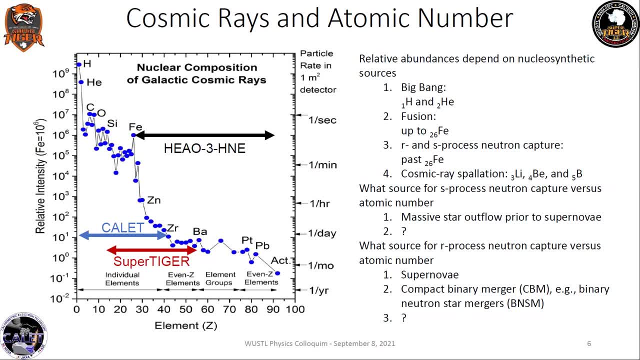 Whereas with rapid it happens very quickly, so fast that neutrons keep adding before there's a chance to decay stability. So you get neutron heavy. you get different isotope production that way, And some elements are predominantly R, some are predominantly S. 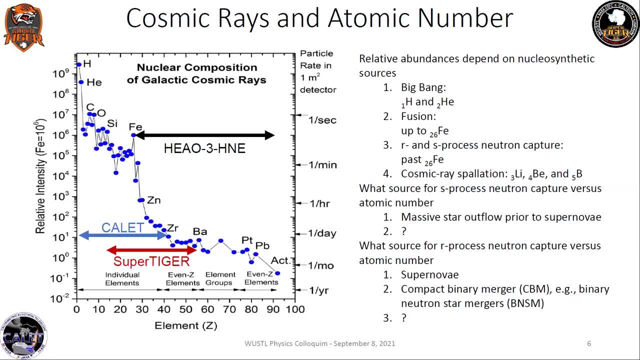 And so, while we believe, we understand that this process is happening predominantly in massive stars during their lives, their process is understood. used to be thought that it was all happening during supernovae, but now we understand the compact binary mergers, including the binary neutron star mergers. 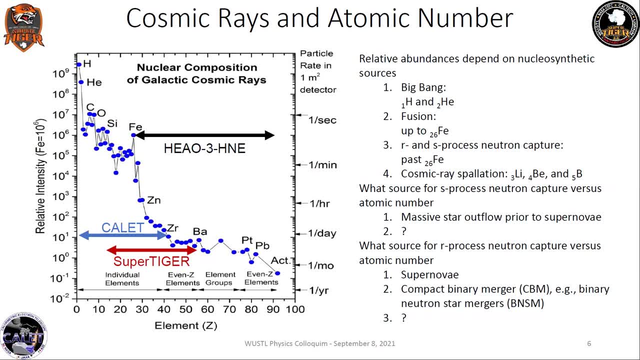 are very likely sources of significant contributions of our process, And so it's the right mixture. and which elements come from which process? And, of course, there's just unknowns. We don't know what all is doing that. All right, so I need to move on to Kellett. 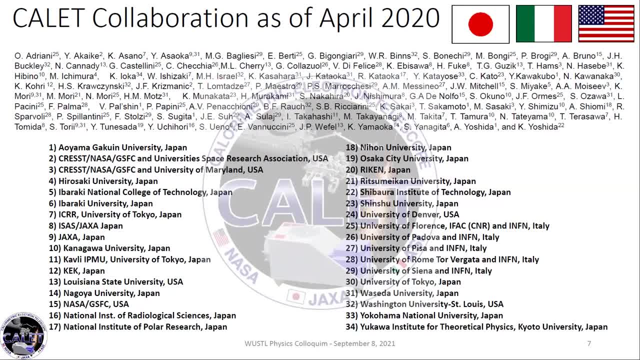 So it's the first and it's what we're talking about in this Kellett collaboration, And this is as of a certain date, because I didn't have time to update it. I didn't want to be misrepresent. the current status. 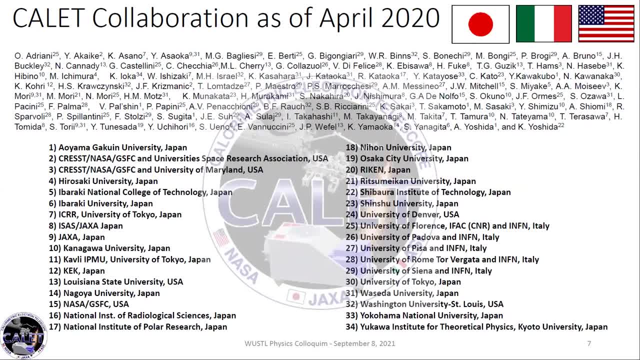 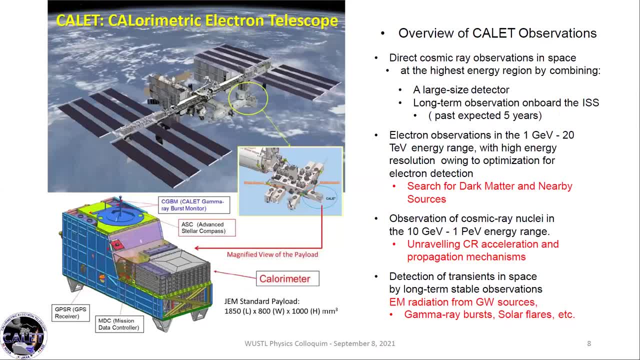 It's a collaboration evolving, led by the Japanese and involving Italians and Americans, And we're Bob and Marty and I are in there somewhere and have Wolfgang. So Kellett is a telemetry electron telescope. This has been said. it's on the international space station. 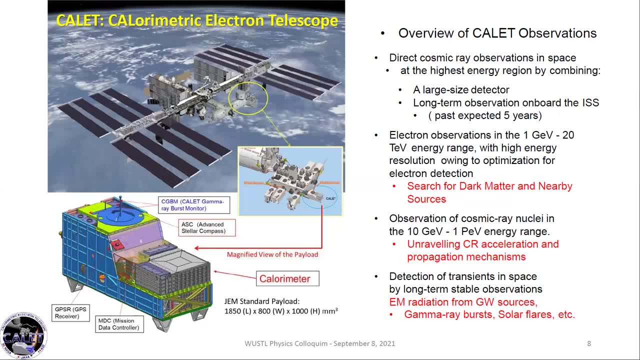 And it is focused on, of course, making electronic observations And it's colorimeter is a specifically designed for electron, electromagnetic measurements, but it also will measure nuclei And again the energy ranges up to one PEV for the nuclei and 20 TV for the electron. 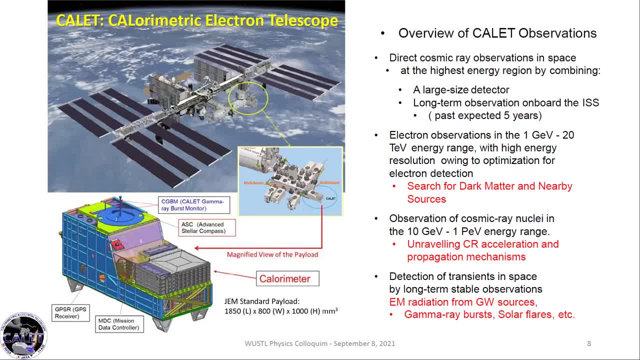 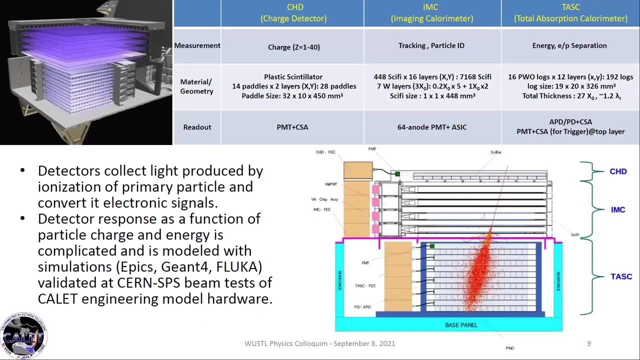 It's also measures gamma rays and looks for coincidence with gamma ray bursts and also gravitational wave sources, solar flares and whatnot. And you can see the palette at the bottom left, just the basic structure of the main color emitters at the front that they're pointing at conveniently. 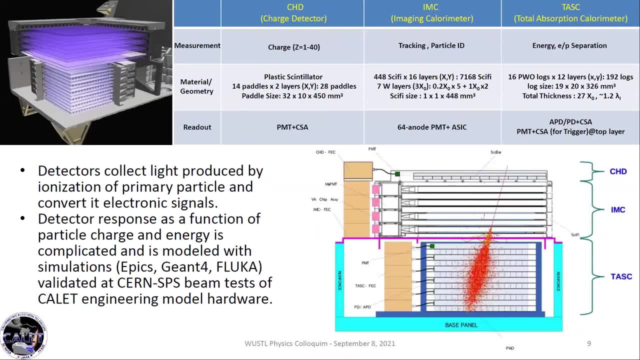 So just a little bit more about the detector. I'm not gonna go into too much, but it has three main components. as the charge detector of CHD at the top It measures the simulators to measure the charge of the incoming nucleus or electron. 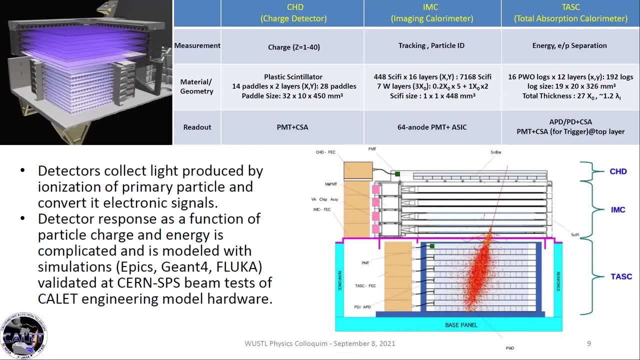 And then below that there's an imaging colorimeter which has multiple layers of simulating fibers, each of which is read out individually, So you can see where the particle track went through. And then, below that is the total absorption colorimeter. 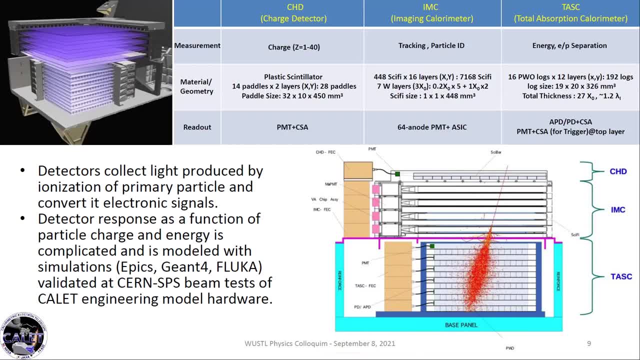 which is the main energy measurement And that captures as much of the energy as possible. There's always leakage with the colorimeter instrument, but it's got good containment for electrons. Now all these detectors work by measuring the light that's generated when ionization energy losses. 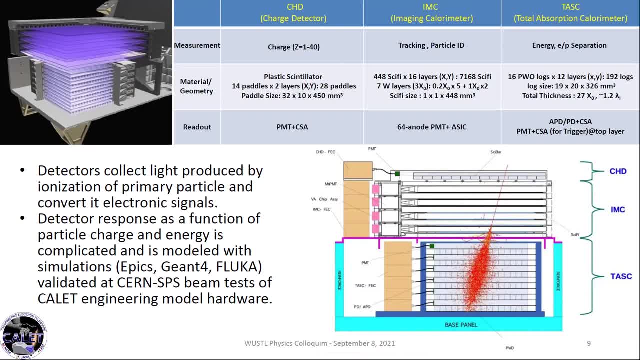 are converted within these special types of materials And the exact characterization of how that depends how this light production is going to change and depends upon the charge and energy of a species- is very complicated And we handled this using models, using simulations- EPICS, JAN and FLUCA. 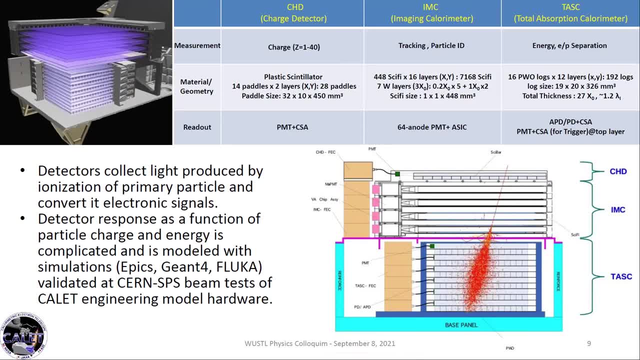 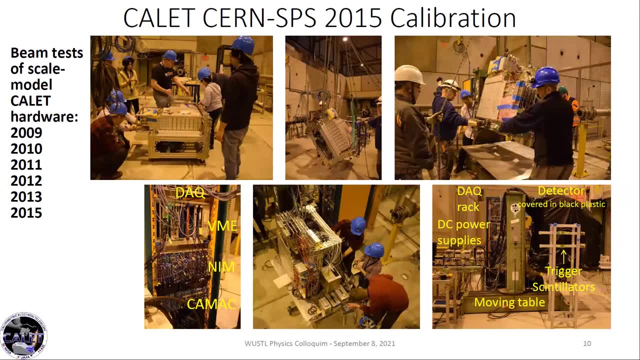 So we use multiple ones to cross-validate that we have tested and validated at CERN. SPS runs. This is kind of what that kind of thing looks like. You go to CERN, the super proton synchrotron in the north area and Prevacent. 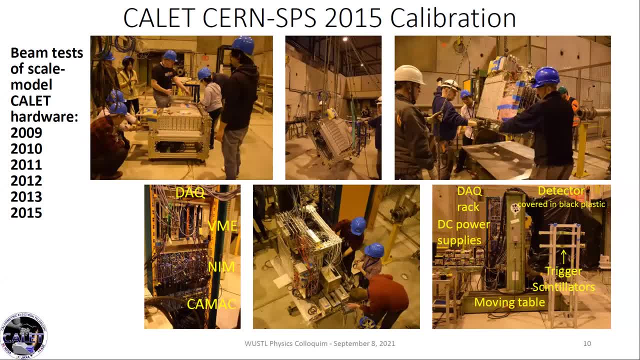 and you set up your detector and you expose it, and you expose it to beams, And we did well. I'm going to show six at least beam tests. I don't know if that's exactly the total count or not. 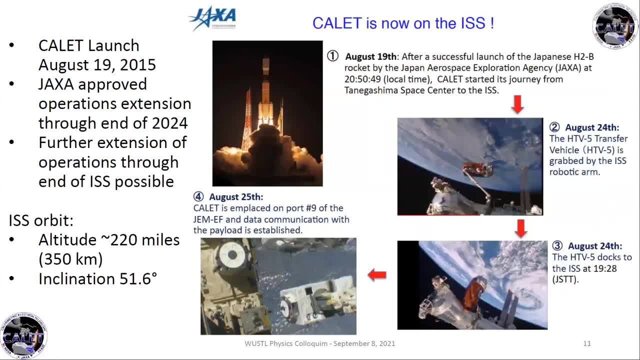 but it's an adventure and an important part. It's a lot of what we do before we launch And then eventually you get to launch. So CALIT launched on August 19, 2015, and has been operating since shortly thereafter. 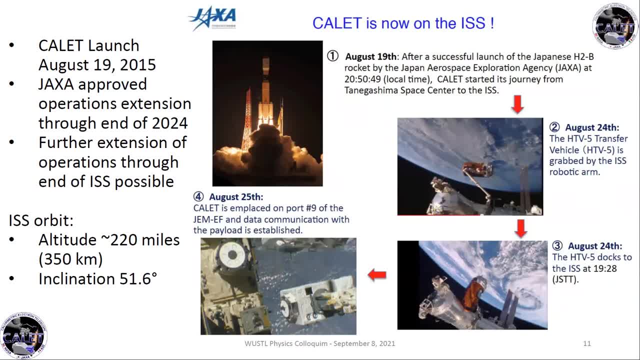 It took about a month or so to get everything checked out. And then the ISS orbits 220 miles. They're at about 350 kilometers, but it of course varies and they have to keep correcting it Every so often, reboosting it. 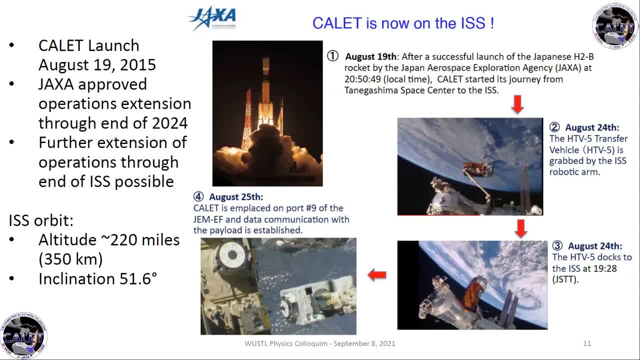 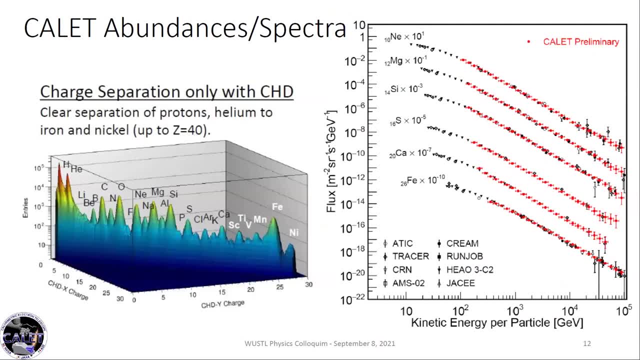 and also reorienting it as the Russians fire the rockets and the things are spinning And the inclination of the orbit is 51.6 degrees, So CALIT. well, you know, I mentioned energy spectra. I showed you the little particle spectra. 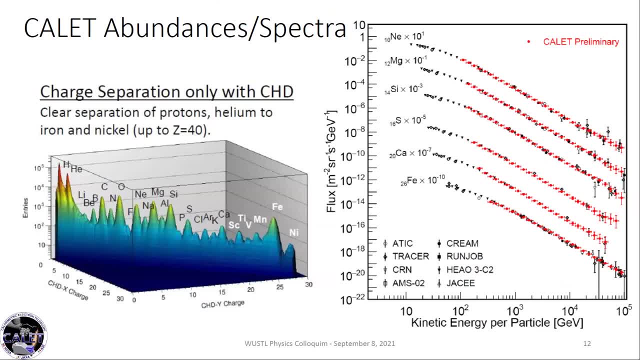 Well, but with the more abundant elements, and you can see a plot in the bottom left showing charge measurement for the CFC charge detector has two layers And so with the plotting, press point X and Y. you see it goes along the diagonal, as you might expect. 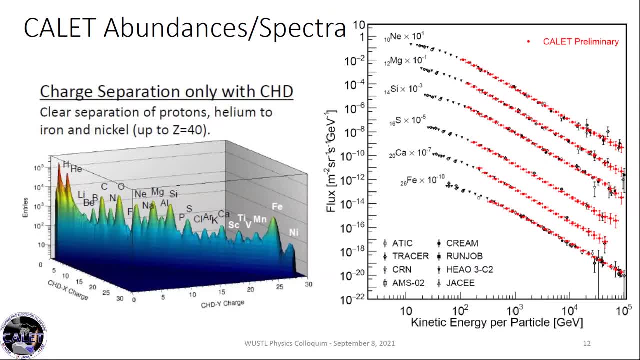 in the three-dimensional histogram here And you see what you kind of expect in terms of the will of the abundances, hydrogen and helium being much more abundant and then things falling off again after iron. But for the more abundant elements up through iron, 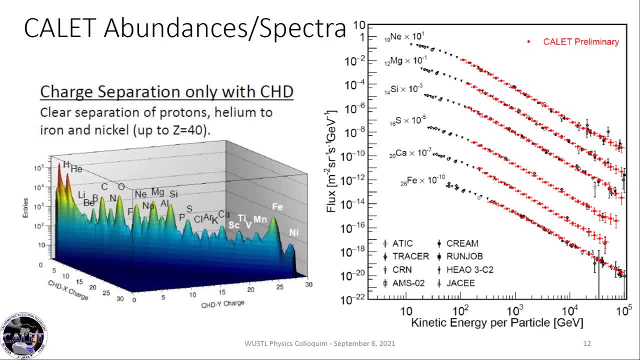 you can measure spectra And so they have shown here on the right plot and they've been a multiply by arbitrary numbers just to separate them out. But you can see that CALIT's made good measurements and comparison with other instruments. This is still a work in progress, of course. 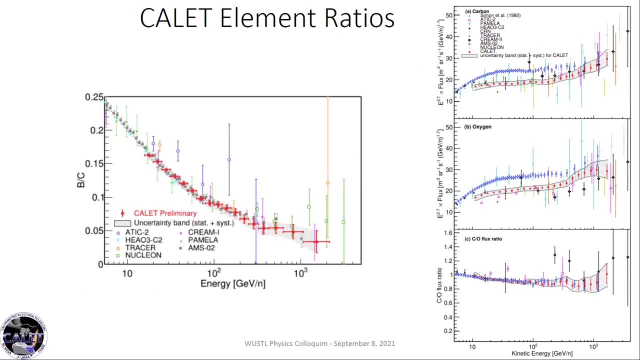 At the ICRC. these are some of the other results of a present. So we have a boron to carbon and that's really important for understanding propagation. As I mentioned, the lightest elements are particularly are produced in fragmentation products. 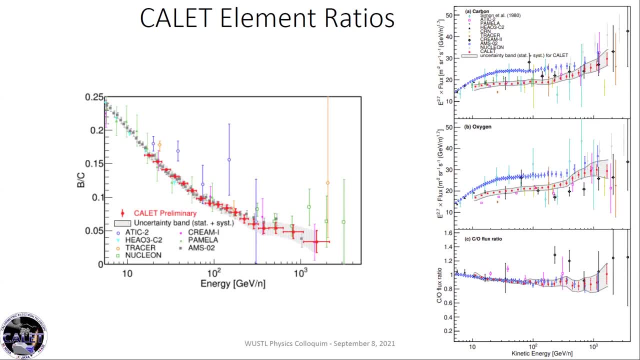 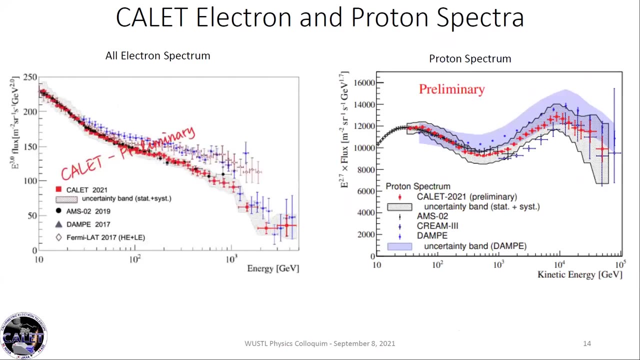 So they're almost entirely, or are entirely secondaries. The boron to carbon ratio helps with that. Also shown is the carbon spectra and the oxygen spectra that go into the carbon to oxygen ratio, which is the measurement shown. So again, the primary purpose of CAL. 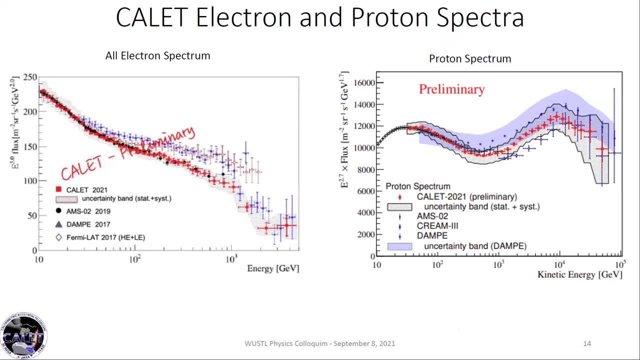 is the electron spectrum and you see they're very careful to put preliminary on everything. But you can see the CALIT measurements are in red, The electron's on the left and the proton spectrum's on the right, And you can see the CALIT agrees with some instruments. 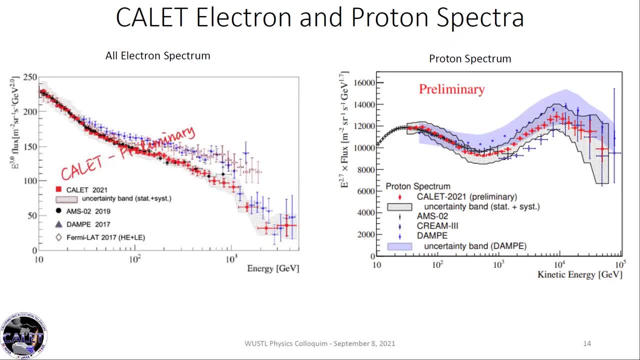 other instruments, measurements, and it disagrees with others. And the fun part is it's not consistently agreeing with the same instruments on the same measurements, Nor does it agree necessarily on the same with the same type of instrument or disagree- It varies with measurements. 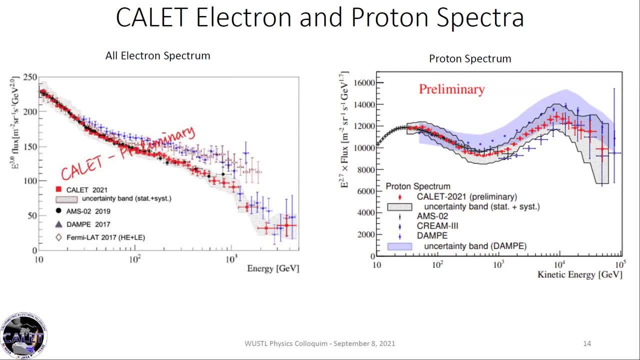 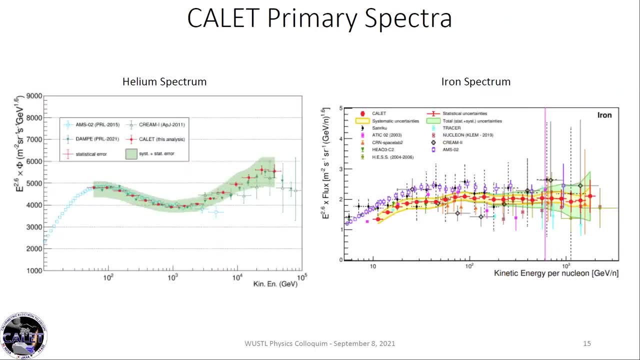 So it's just there's a lot to understand with this, and that's why it's good to have multiple instruments making the same measurements And then some other- okay, Helium and iron spectra, And so you know one of the interesting features. 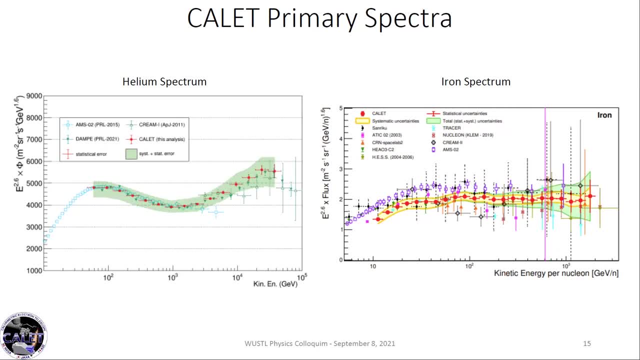 of the high energy is the spectra kicks up again, which is not expected, And that's seen in a lot of spectra, but it's not seen in iron. So that's one of the more recent publications, for KELA is showing the iron spectra is not showing this. 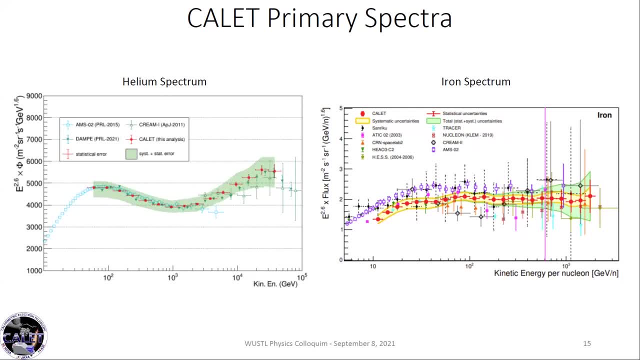 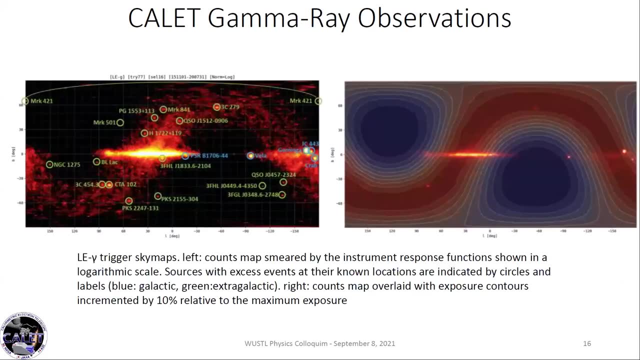 this kickback up with the highest energies. So there's some clear difference And a lot, of, a lot of spectra seem to have that feature at the lower charge, Lower atomic numbers. So it's telling you something I mentioned that KELA also does make gamma ray observations. 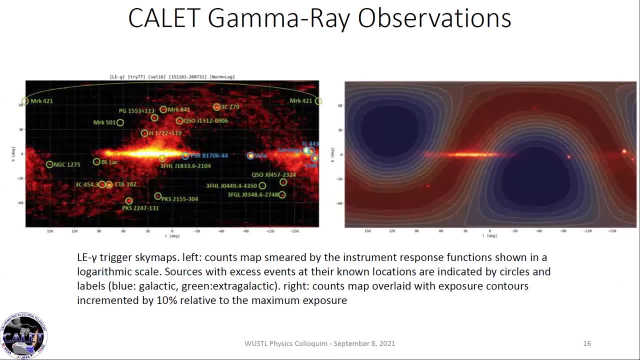 And so I pulled this from the latest ICRC where you can see the galactic plane. You can see numbers of sources seen way back at the beginning. The very first meeting I went to, I did an estimate of the gamma rays that we would expect to see. 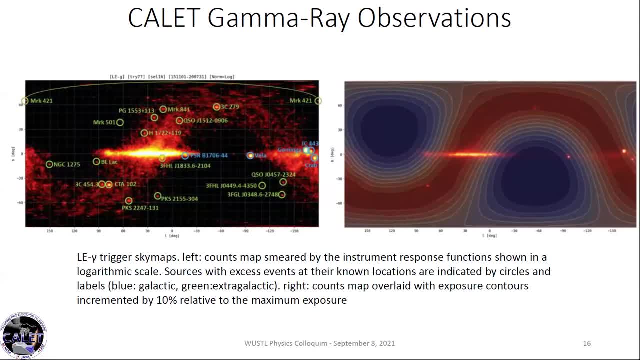 And it was not very encouraging. I thought we'd only see the few most abundant, the brightest sources. But fortunately a grad student at LSU, now post-doc, had got it And it was very encouraging. I thought we'd only see the few most abundant, the brightest sources. But fortunately a grad student at LSU, now post-doc, had got it And it was very encouraging. I thought we'd only see the few, most abundant, the brightest sources, But fortunately a grad student at LSU, now post-doc, had got it. 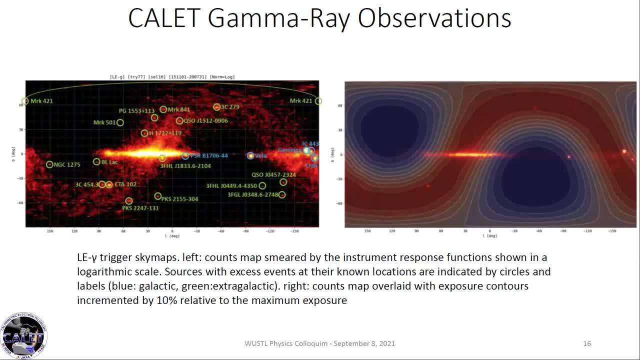 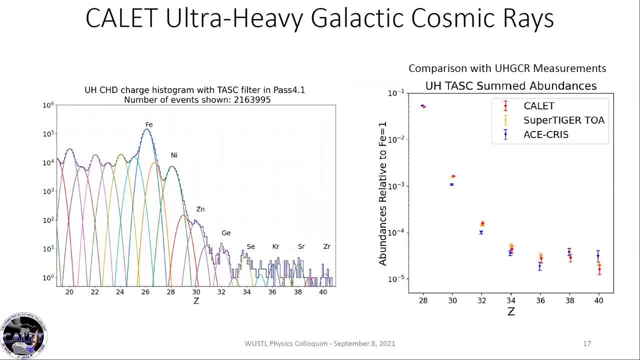 We did a lot more work And you can see that they really can observe significant sources and the diffuse background. So the focus of WashU, though, as always, is on the ultra-heavies, the rare elements beyond, well, really, nickel, but beyond iron. 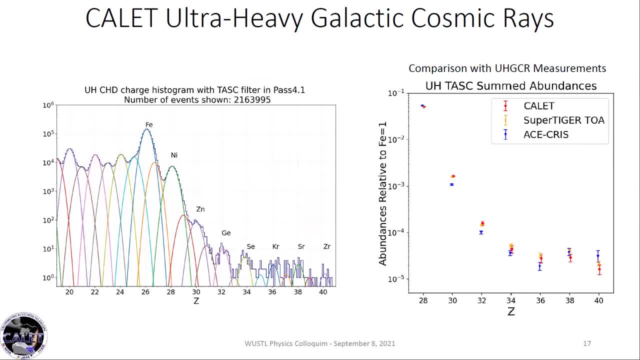 This is work of Wolfgang Zober, which I really should have just explicitly put on there. I should have actually called everyone out. That was oversight and my haste of throwing this together. The histogram on the left is what he showed at the ICRC. 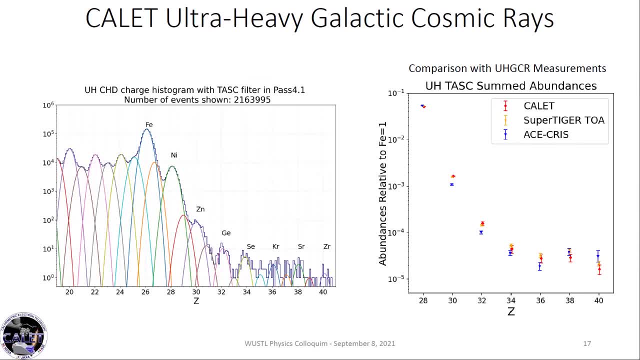 And you can see that his analysis is really beginning to show some good resolution out in the ultra-heavy range. And then comparing on the right with other measurements for the even elements of the paired abundances, Well, I could speak up, but is it even or pairs? 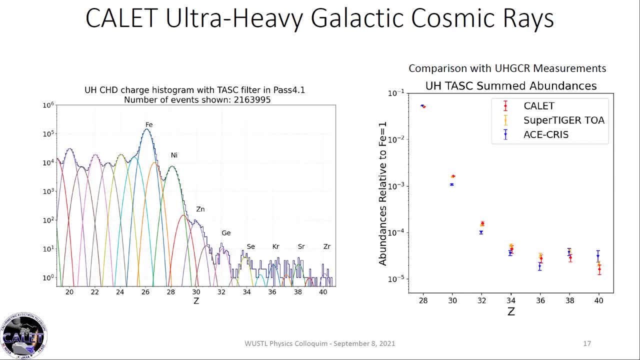 It's pairs on the left. Yeah, OK, That makes sense. Anyway, you can see that with this preliminary- and he's working to get individual elements- the odds are even separate, both resolved And it looks promising. anyway, You can see that we have reasonable agreement. 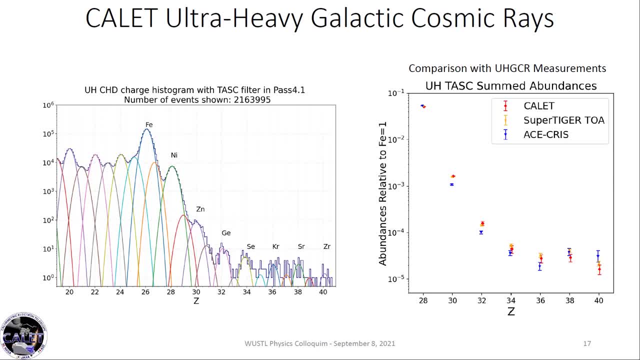 with the super-Tiger measurements we'll be talking about soon, but also with the ACE-CRIS measurements that have been made, And that's Bob Benz and Marty Israel's current effort is focused on the ultra-heavies there. OK, moving on to super-Tiger, because I probably 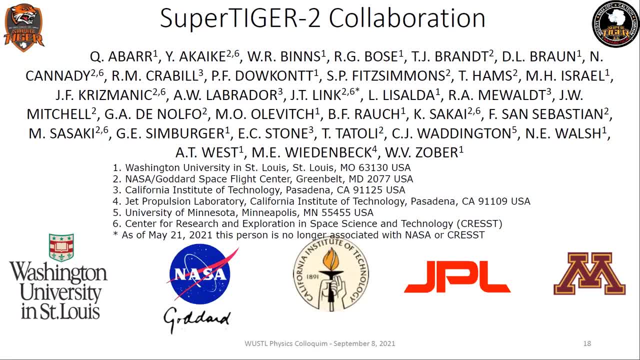 can't speak too fast with the way things were. So this is the super-Tiger II collaboration, or at least the most recent iteration of it, And we've lost our Minnesota colleague in the last couple of years. unfortunately, Jake Waddington passed away, but we're. 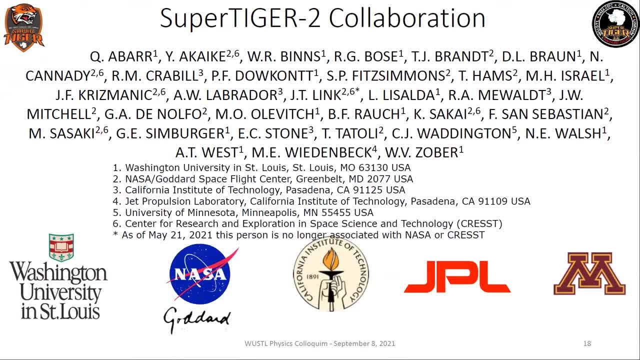 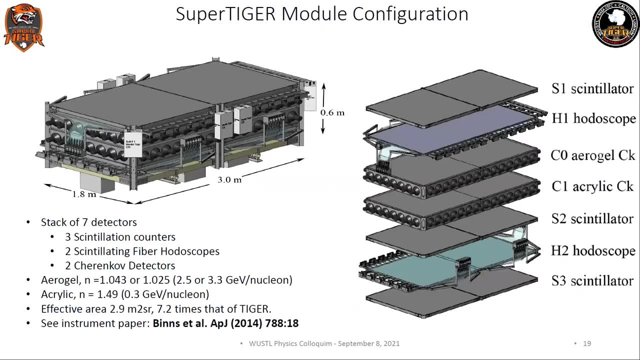 going to continue to have him And we've had a lot of bonus graduate student participation and helping us. that I'll point out later. It includes not just Wolfgang and Nathan, who's now postdoc, but also and Andrew West. All right, so just a little bit about super-Tiger, which. 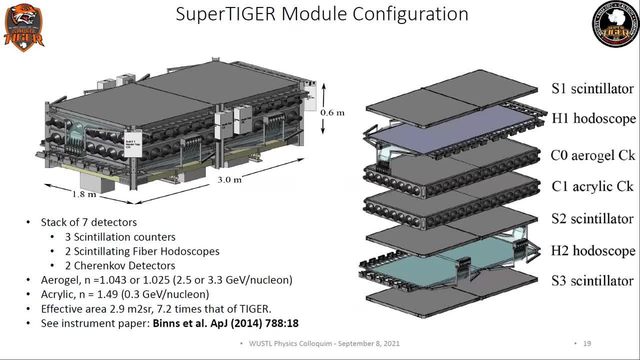 many people will have already seen, Super-Tiger has two modules, And so I'm showing pictures of a full module on the left and an expanded view of a module on the right where you can see all the detector components. You can see it's a stack of seven detector types. 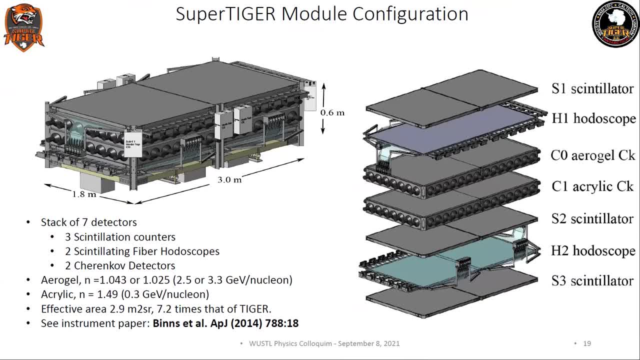 And there are three scintillators spread throughout top and bottom and underneath the trinkets, where there's an aerogel and acrylic, And also near the top and bottom. you have hodoscopes, HODOSCOPE planes. 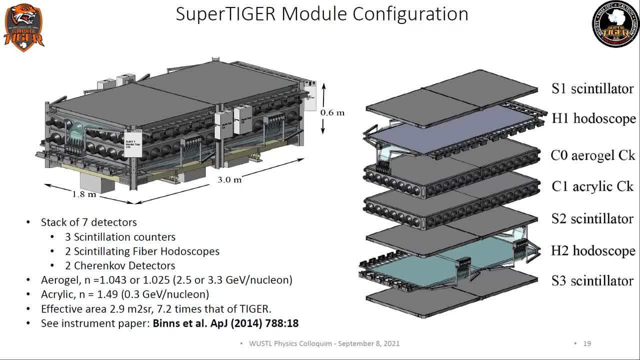 HODOSCOPE, scintillating up the fibers that give us trajectory and position, and the instrument which is vital for making corrections for instrument effects. That's, in fact, what graduate students spend most of their time doing is instrument-level corrections. 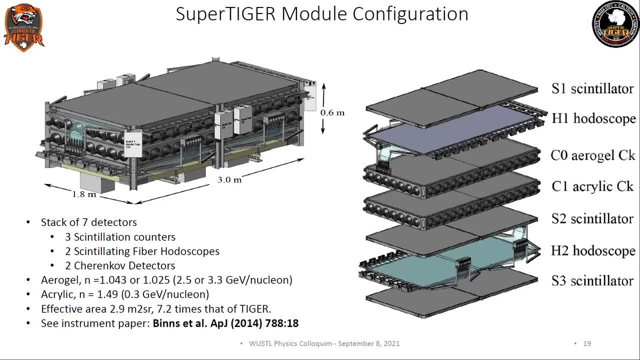 and to the analysis, to get to the science. The science is the last minute, end of the road. All of a sudden you're there, kind of magical moment. But the scintillators, they measure the light that is from ionization. 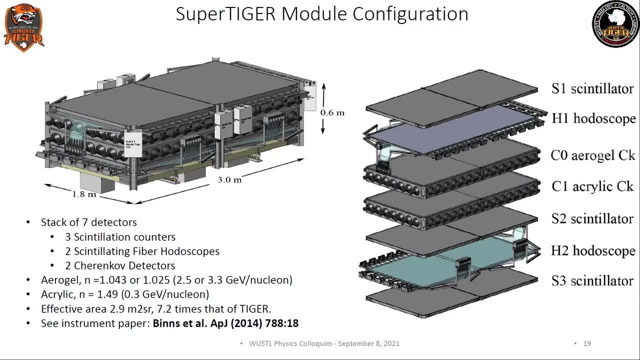 But the Trenckloff detectors. that's the electromagnetic shockwave you get when you have a charged particle traveling through a dielectric medium at greater than the local speed of light. And so the threshold is related to the index of a fraction inversely related. 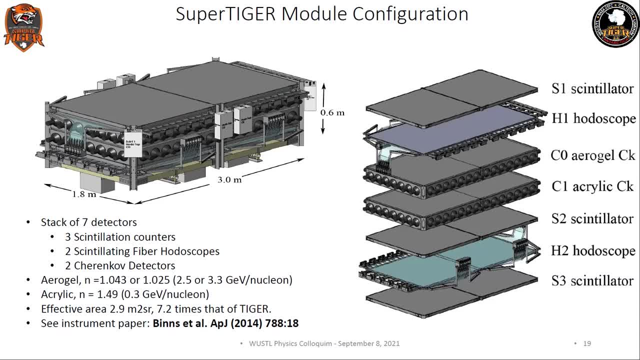 And so we have two different materials. You have acrylic or plastic, which is about 1.5.. So it turns on about 2 thirds the speed of light, And then an aerogel, silica aerogel, so it's a kind. 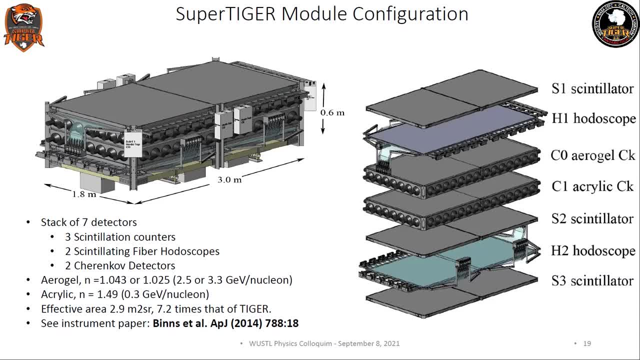 of solid smoke, Very thin material, that is 1.04 or 1.025. And so that's very much closer to the speed of light before that turns on. And so that combination of detectors allows us to measure charge and velocity, which correlates. 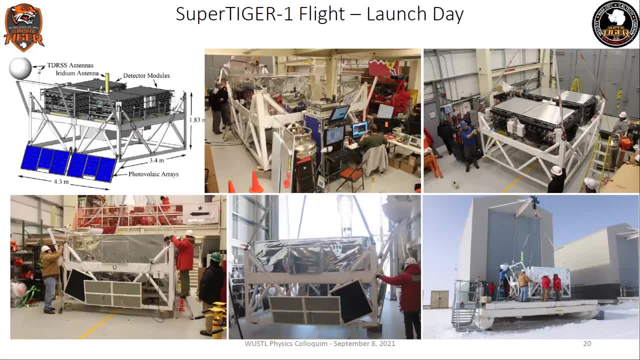 obviously very directly with energy And I'm not going to go into the full details of the analysis. I'm going to show results, But first and foremost we'll go through the flights. Super Tiger I: the first flight was record setting. 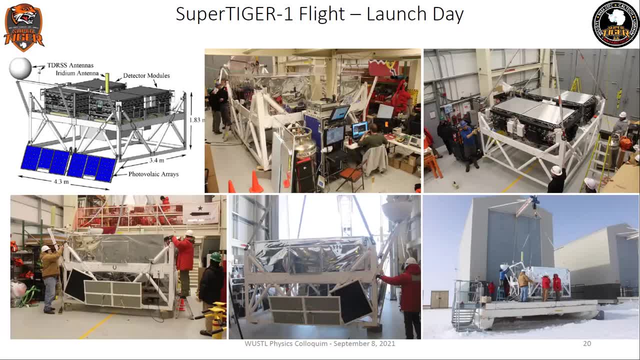 Got 55 days. You can see the full instrument model there. on the upper left You can see the two modules on the gondola, power, solar panels up front and antennas. And this is just what it was like working in the Caleb. 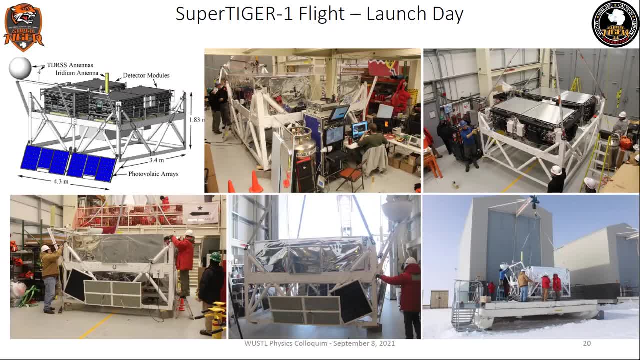 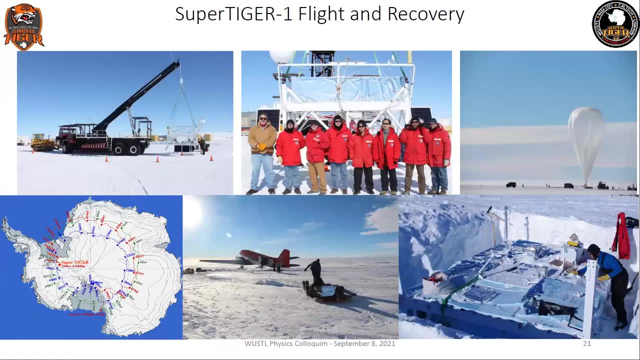 building in McMurdo. I wasn't there. I just got to monitor the flight for 55 days and do commanding from up here. You can see this pack of folks here in the upper center were the ones who deployed, including Bob, And you can see at launch. you can see the inflation. 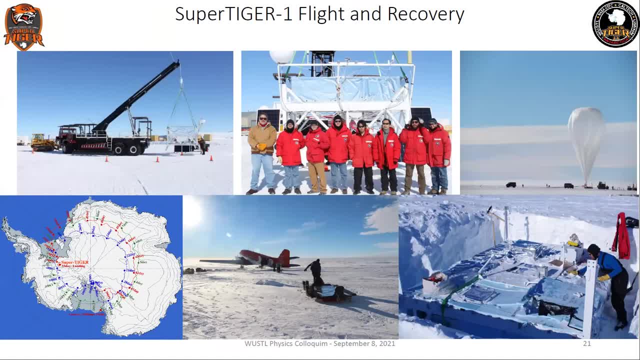 Those are vans in the foreground. You can see the tractor there as well. So it's a very large balloon. Once inflated, you can put a football field inside of it or have the Statue of Liberty stand inside of it. So it's a big balloon lifting a really heavy payload. 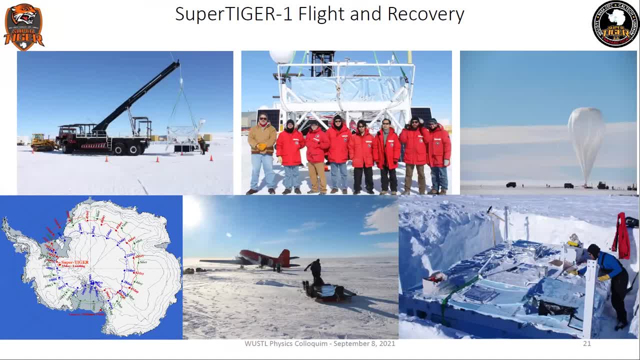 You can see the size of the payload, up to 6,000 pounds. The bottom left you can see the track. It went around the continent two and 2 3rds times. It's a shame it couldn't quite go any farther, because we're 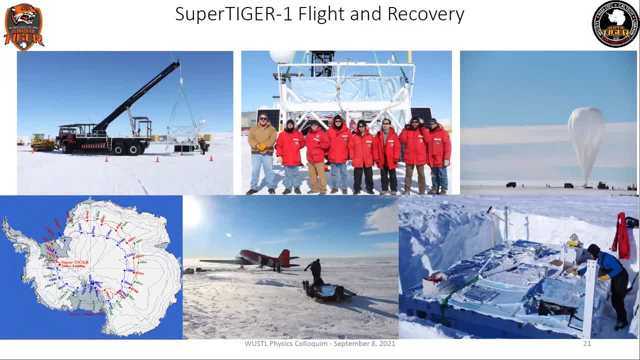 getting close to the end of life determination battery and didn't want to risk letting it go any farther, And so the experiment flew set a record: 55 days. It has not been broken for heavy lift zero pressure balloon and might never be broken. 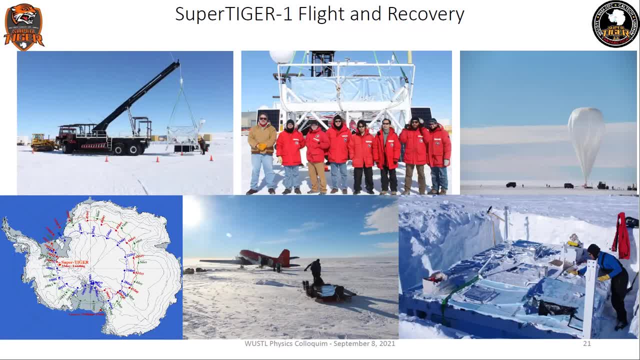 You never know, of course. You say that kind of thing and then someone will break it, And then it had to be recovered. And it was recovered after two years because, well, the next season there was a government shutdown, And by the time it was recovered, you can see Tom. 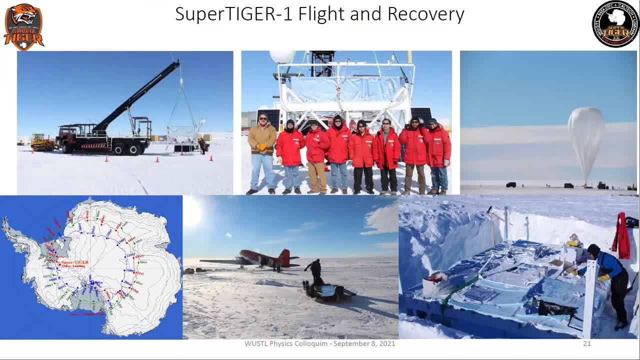 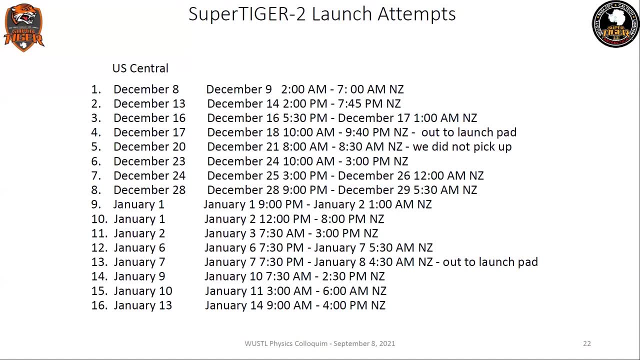 as Ham's collaboration member, now NASA administrator, working to almost single-handedly dig it out with the help from the recovery groom team. But it was successfully recovered. So now we move on to SuperTiger 2.. And we had quite a bit of adventure. 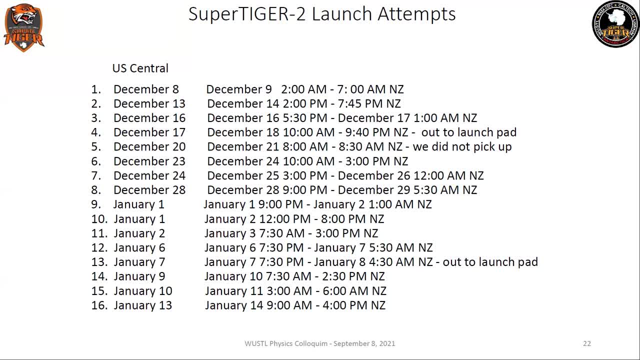 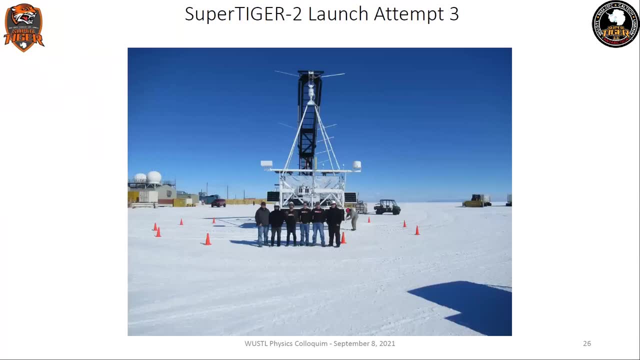 We had in the first season. OK, that was good. First season we had 16 launch attempts without any successful launches. Hang test, we're all looking fresh. One launch attempt, two launch attempts, two launch attempts, four launch attempts. 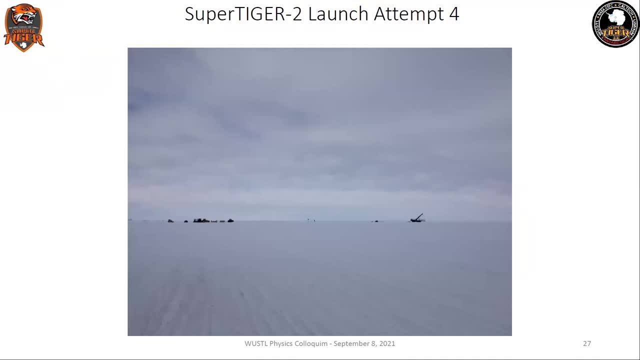 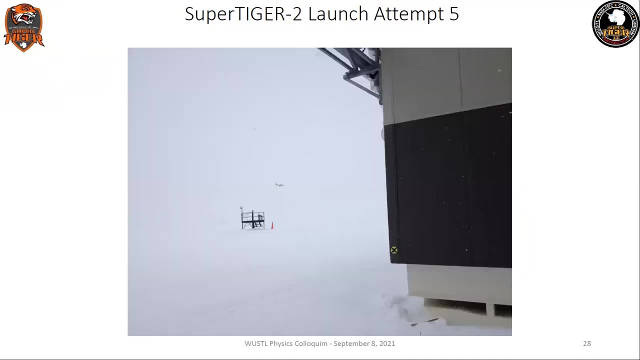 We got close. We actually were on the field, We were about to lay out And if we had laid out it would have been really hard to not launch, because it's hard to put the balloon safely back in the box without tearing it. 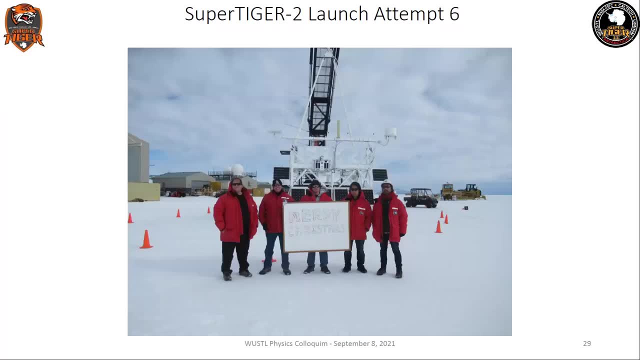 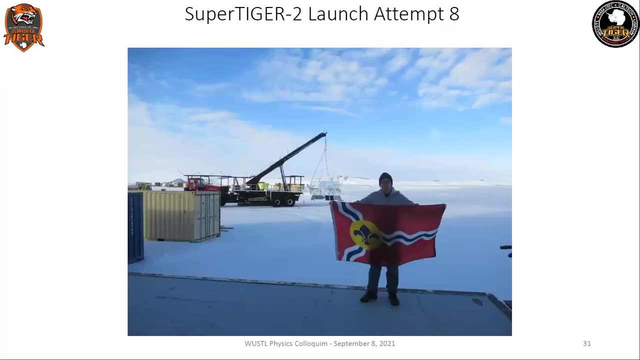 Fifth launch attempt was barely a launch attempt, And now we've made it to Christmas And you can see the group is shrinking. And seven launch attempt, oh eight. Here's Richard Bowes. You're representing St Louis, as you want to do. 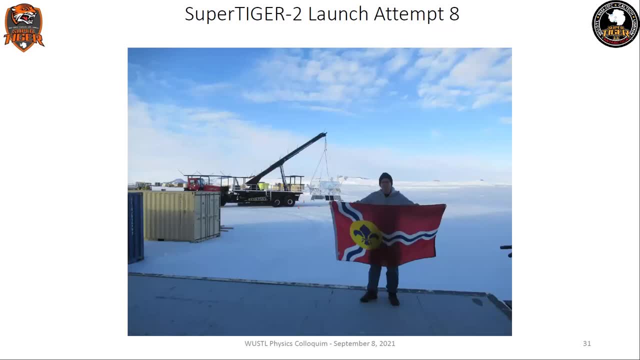 And that's how he of course gets to have Richard Bowes Day be June 5th. He gave the flag to the mayor And the mayor appreciated it. Oh, now it's New Year's And you can see the group's got even smaller. 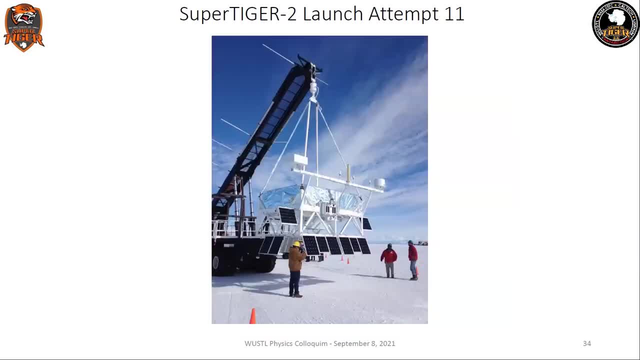 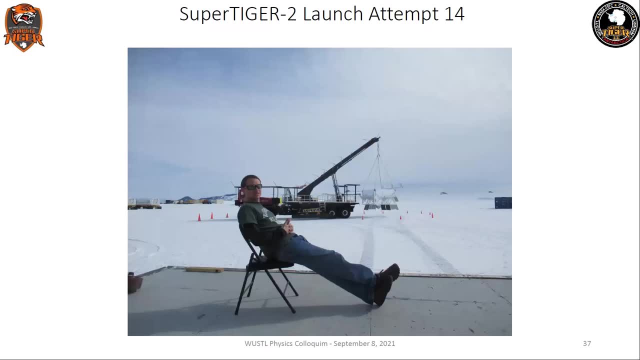 We're down to four. It's a warmer day. 10th, 11th, 12th, 13th- Well, we actually were rolling a bit. 14, well, it was a really good day. We were on the deck. 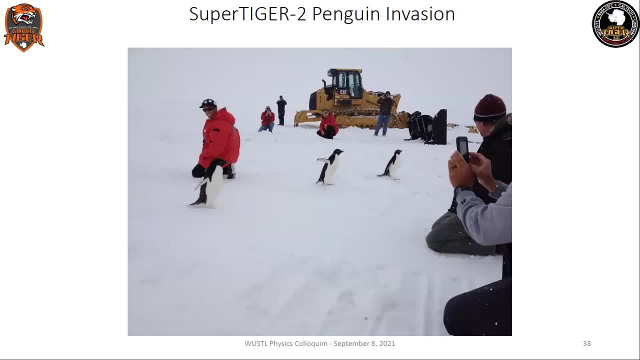 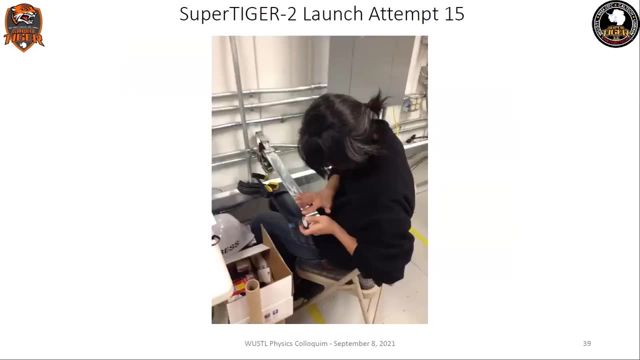 Oh, and I was there for the penguin invasion, So there was a benefit. I was the person who went out there every day. A lot of people would hang back in McMurdo when we weren't having launch attempts, But because I happened to be there, I could see the penguins. 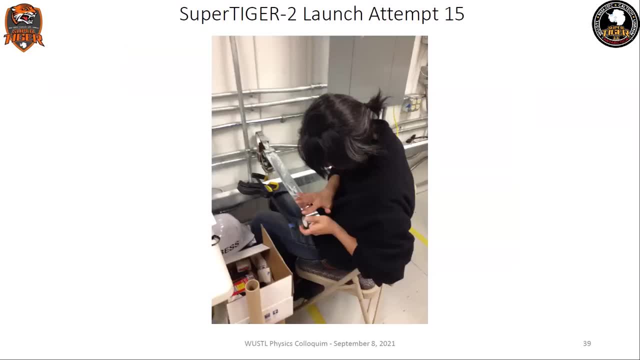 The 15th launch attempt, we ran out of the wider tape. And so, Kenichi, here, Dr Sakai is making the wider tape out of three rolls of narrower tape Launched on 16.. And then we gave up and packed it in. 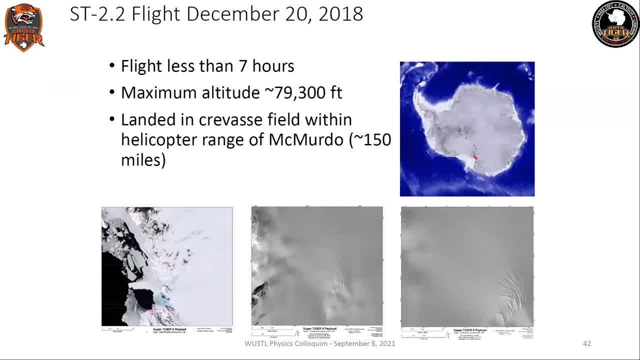 Well, the next season, we came down And we got a launch on December 20th 2018.. But the flight was less than seven hours. We couldn't clear 79,300 feet. We had a leaky balloon. 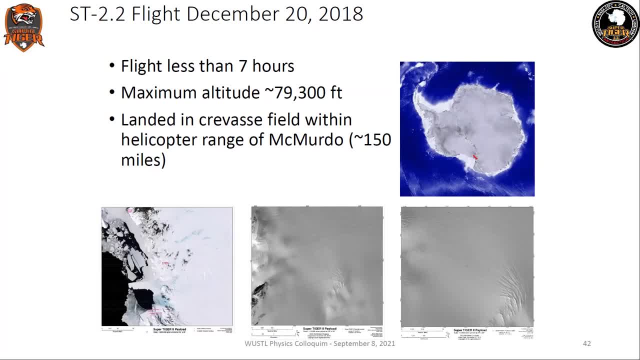 It came down so fast that they didn't have a lot of choices. Once it goes below 60,000, there's an automatic termination system. And where it came in, it came in into a crevasse field. You can at least see the fingers of the crevasses. 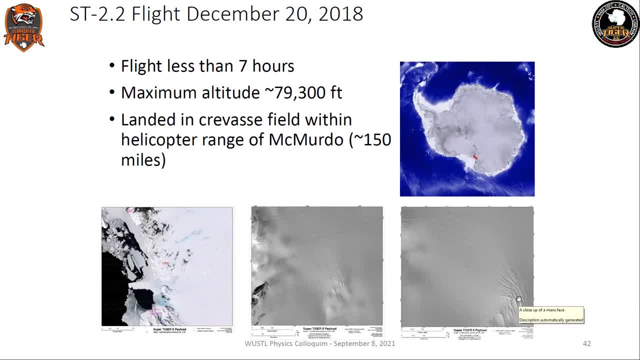 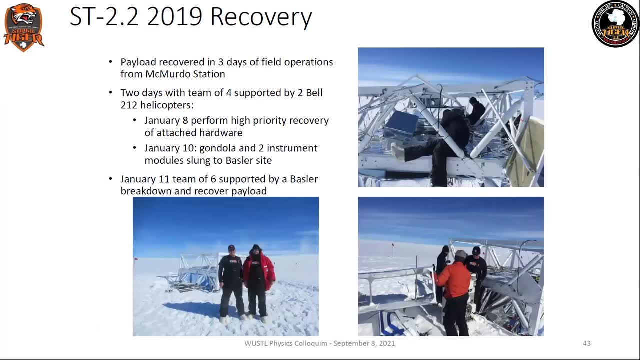 in this bottom picture, if you look hard enough. And I landed square In the middle of that crevasse field. So that was a real adventure to recover it. It took three days of operations. First few days we used two helicopters. 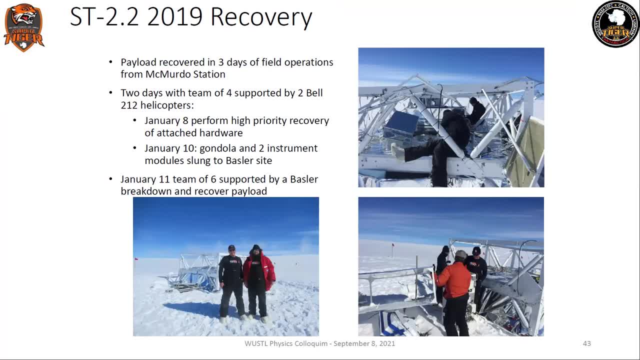 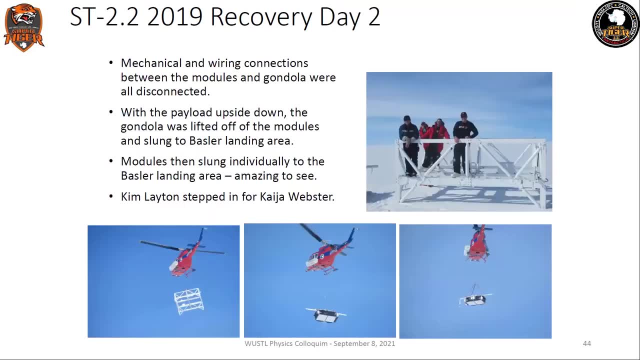 to first fly out there and get all the loose, easily removable things off the gondola, And then the next day we had the helicopters disassemble the major components and carry them over to a compression zone where an airplane can safely land, And then we got off the ground. 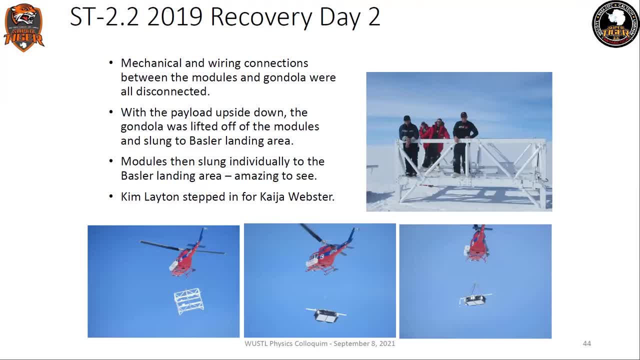 And then we got off the ground. And then we got off the ground, Which was really quite epic. I'm glad it worked, because it was my idea to lift the gondola off of the instrument, And I'm glad they didn't wreck it. 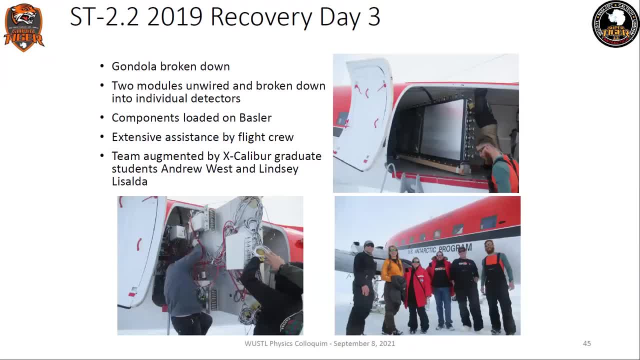 Then on the third day we went and disassembled it all and somehow got it in the plane- the Basler- there in the allowed time on the ground, And that couldn't have been done without the help of Andrew West and Lindsay LaSalda in the field. 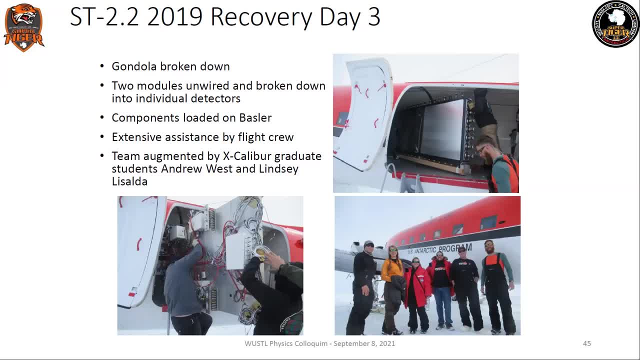 And I love this picture on the bottom right because we're all smiling. But there's another picture I was taking just before. when we were looking at it, We were looking toward the tail, where we're not. The only person smiling was Lindsay. 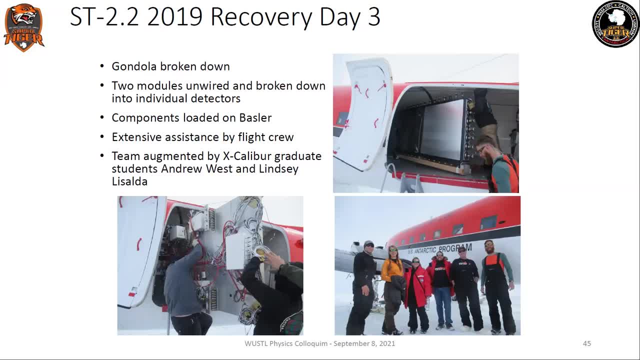 She was a real trooper. that way, The rest of us were looking as worn out as we feel. For those of you who've come to the department, there's now a TV on the second floor, by the elevator, that cycles through lots of pictures. 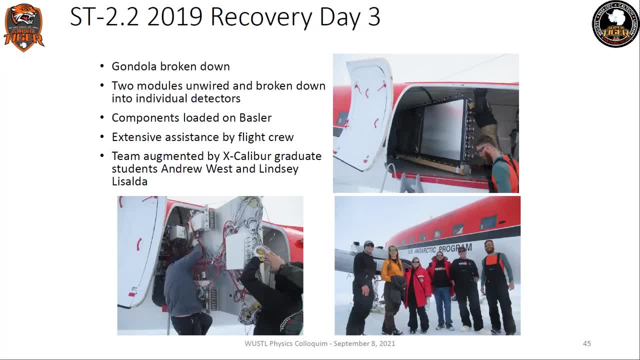 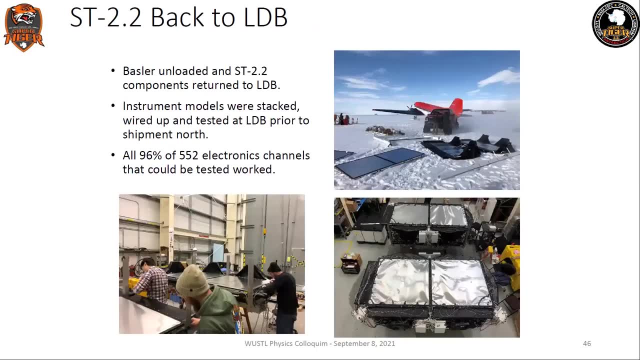 from all the balloon programs, including Spider, Now that we have Joanna Nagy here And you can see those people that I'm talking about. So we had to get it back to LZB, We had to reassemble it, We had to test it to show that it was in good enough shape. 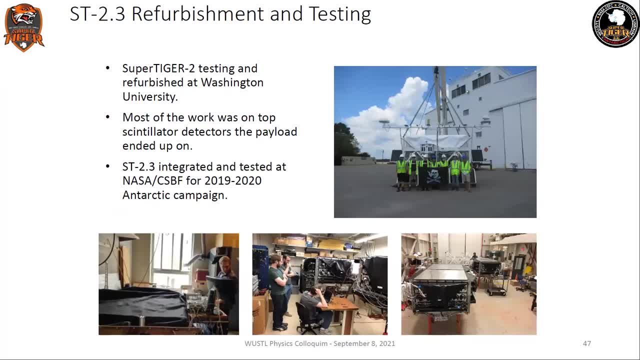 to come back and fly the next year. We had to go through integration again. We had to refurbish it. We had to get help with new grad student support And you can see both Wolfgang and Nathan in the bottom pictures. We got it ready, took it to Antarctica. 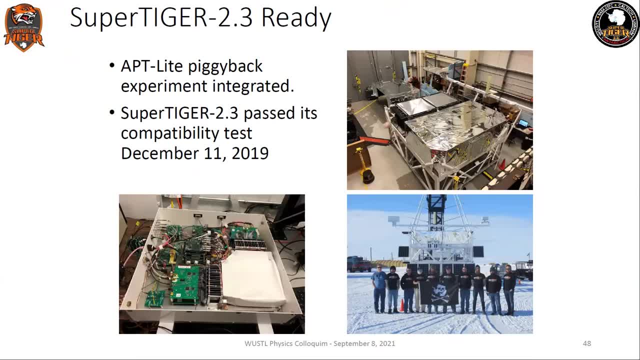 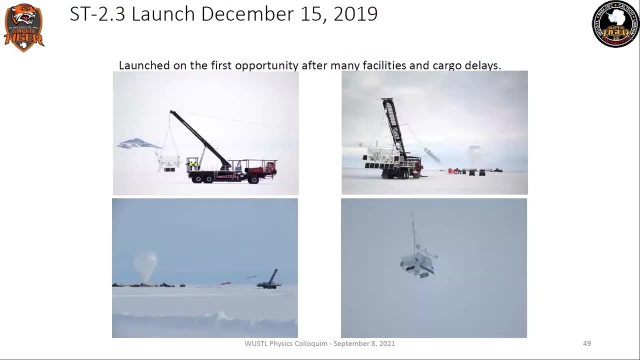 This time we added the APT light piggyback, which was integrated with the payload underneath it, collected data that also was cross-triggered with Super Tiger events and analyzed, And that's it, Thank you. Thank you, This has been published and has gotten Jim Buckley. 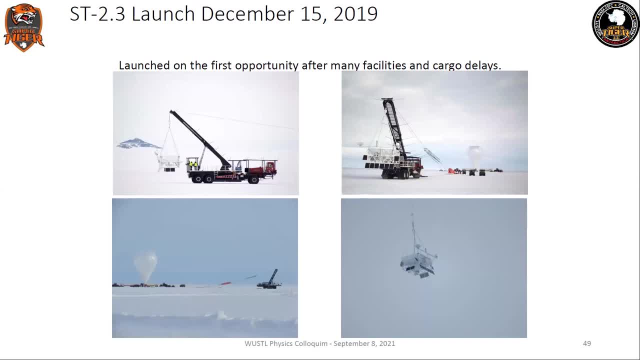 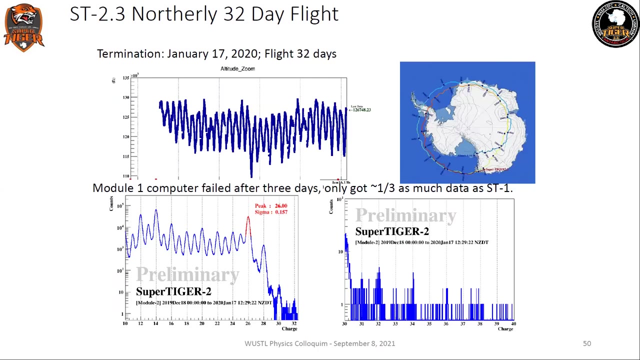 his own balloon instrument called ADAPT, Antarctic Demonstrator of APT, which is, I won't say APT, and get it wrong while he's listening. OK, so we actually got a launch again this time, And this time we got a flight. We got a full 30 days and around the continent twice And we spent an awful lot of time to the north and over the water, which is very scary. Our altitude profile was reasonable, but it dipped a whole lot more when we were over the water. 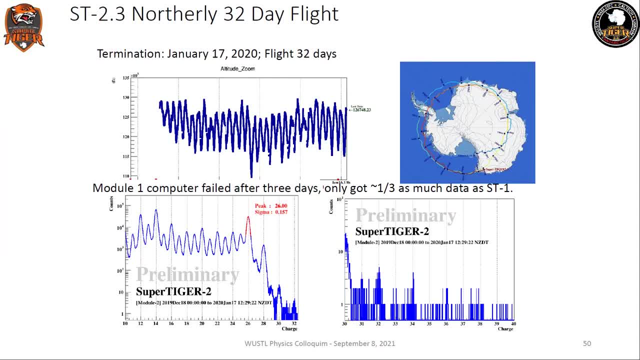 There's also albedo, And the albedo, the light shining off of the ice, heats the balloon and keeps it up higher. And, most significantly, one half of our instrument failed after just three days, And so, even though we had 30 days of flight, which 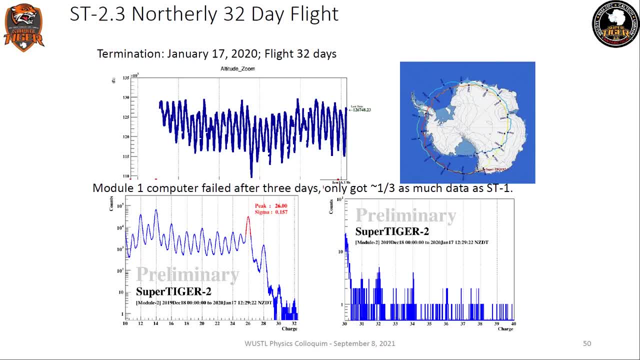 is a significant fraction of 55 days. when you also take a hit on losing one of your models, You get a lot less data. So our data for the SuperTiger 2 flight, which you can see the UH range is pretty sparse. 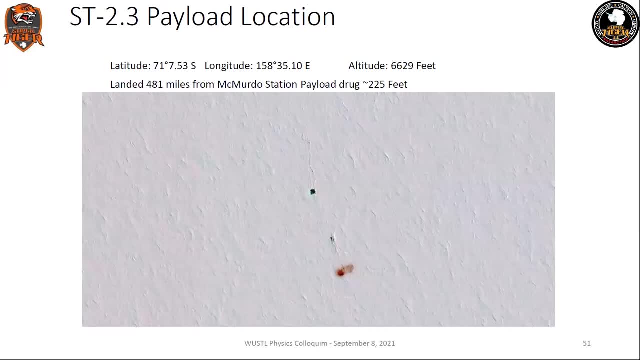 And it's very sparse compared to what we'll see for SuperTiger the first flight. So with the status and payload and it's still here, It's not been recovered. Now we have COVID-related reasons why it's stuck on the ice. 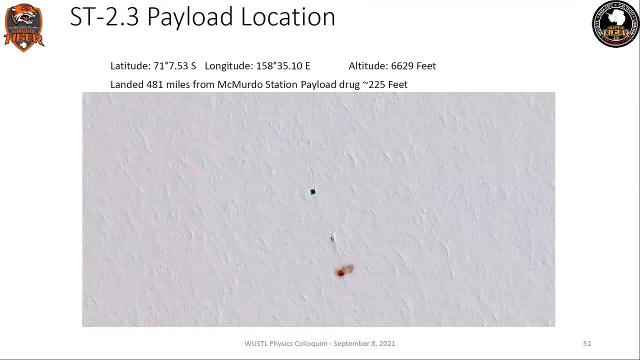 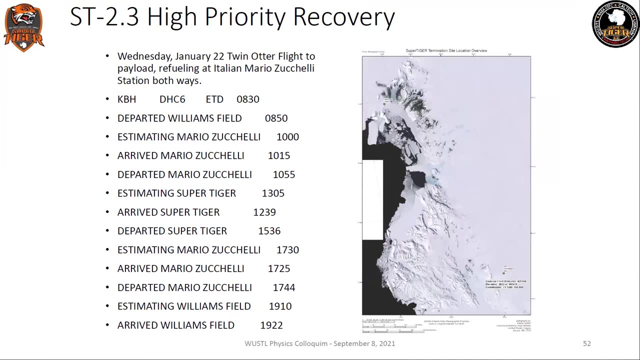 And I'm hoping that next season- not this upcoming season, but a year in 2022, I hope to be able to go down there and pick up our litter. All right, Let's recover it. We did get a high-priority recovery, which was fun. 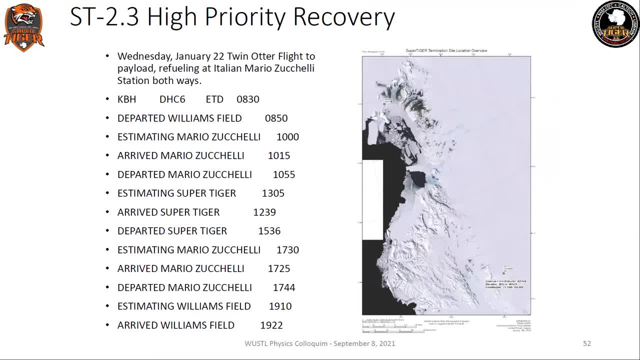 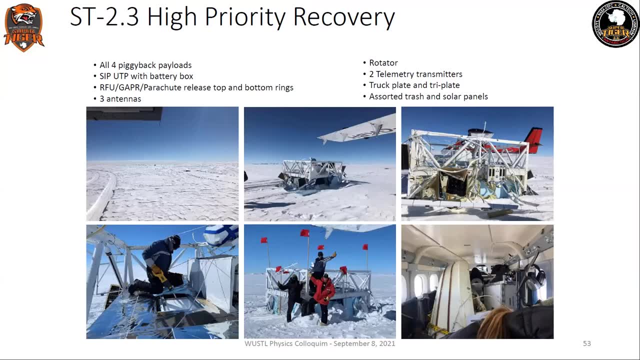 We went through the Italian Mario, the Kelly base, coming and going to get fuel, And we managed to pick up a lot of important pieces, including APT light, which was important for Jim to be able to do. Jim and Zach, Zach Hughes, who got his PhD in part analyzing APT light data. 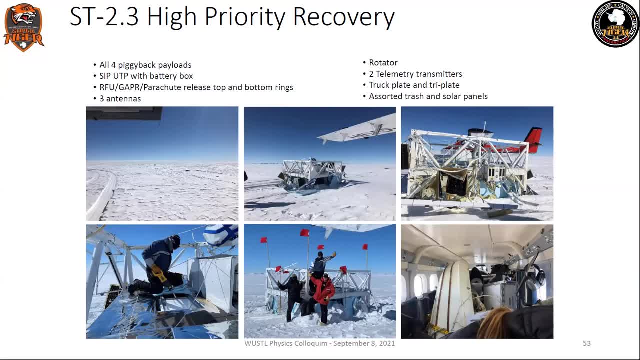 And also the Bass piggyback experiment that collected air samples, sent for Alex Metric on the fourth floor, and then two others that are from other institutions: EMIST and PMC. Turbo Polar Mesosphere Clouds, Turbulence- is what that one stands for. 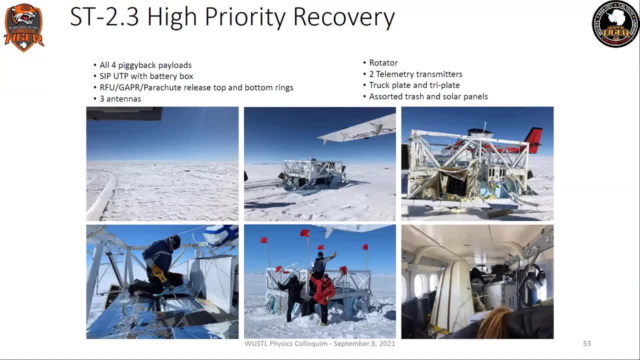 And EMIST is exposing microbes in the stratosphere, which is meant to be. it opens trays that have bacteria on it and exposes them for different samples for different lengths of time, Because the stratosphere is apparently a good surrogate for the surface of Mars. 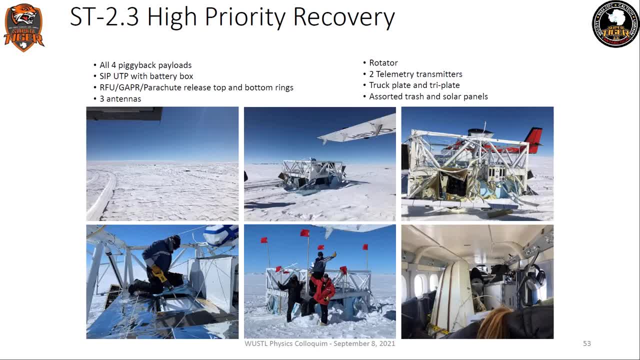 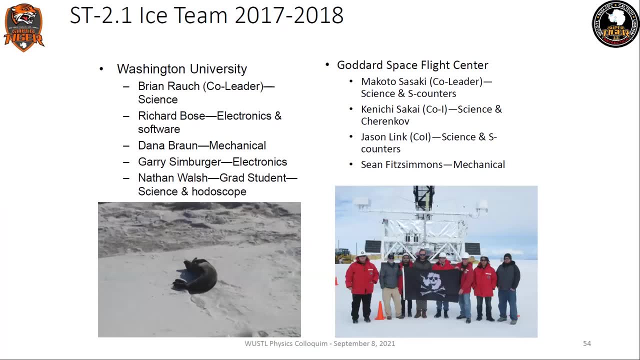 in terms of pressure and radiation environment. At least that's how they do it. That's how they sold it flying on the NASA balloons. This is just a little bit of fun because I got a seal, So there's some wildlife And you can see that the group evolved quite a bit. 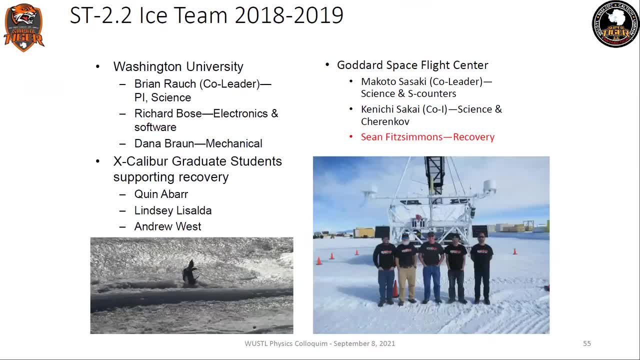 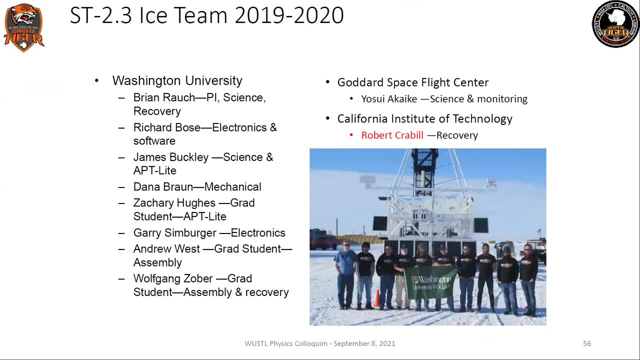 from the first season to the second season- That's a nice little penguin shot there- To the third season, where it was almost entirely washy by the end. We had one person from Goddard in the final year And you can see Jim Buckley there. 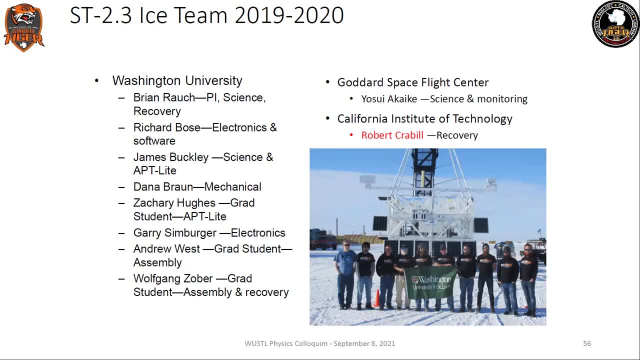 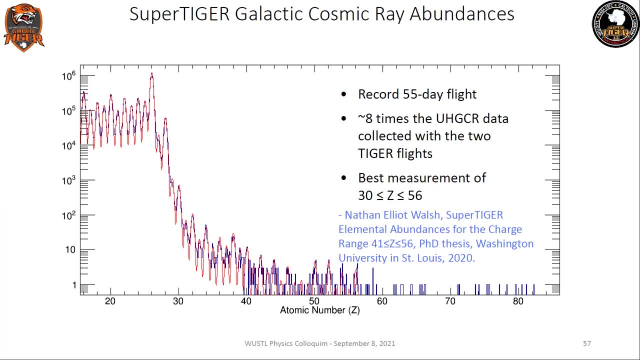 You can't make out that he's got an APT on his shirt, but he did a thing to represent All right. so it's not all just launch attempts and recovery and penguins and whatnot. There's actual real science to be had out of SuperTiger. 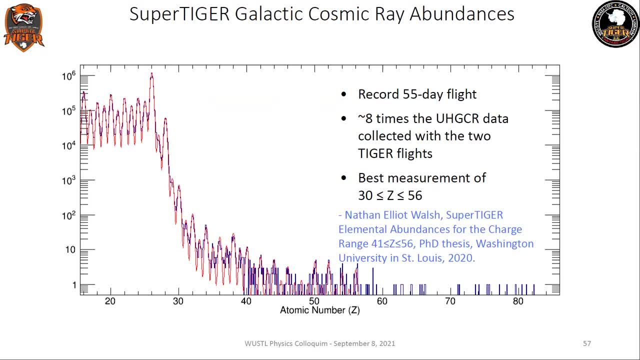 And so Ryan Murphy got his PhD doing SuperTiger analysis through zirconium, through CHARGE40.. And what he found was his SuperTiger measurements agreed with the tiger measurements I got my PhD on, although with far, far better statistics- over eight times the statistics. 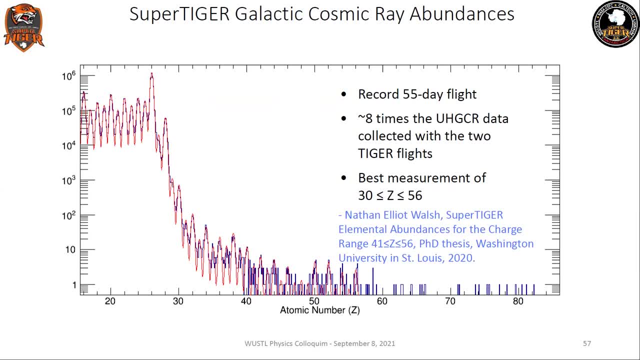 But the real interesting advance here is: Nathan Walsh has analyzed evidences all the way to barium, which is CHARGE56. And you can see here the red superposed fit on top of the histogram. An enormous amount of work has gone into getting here. 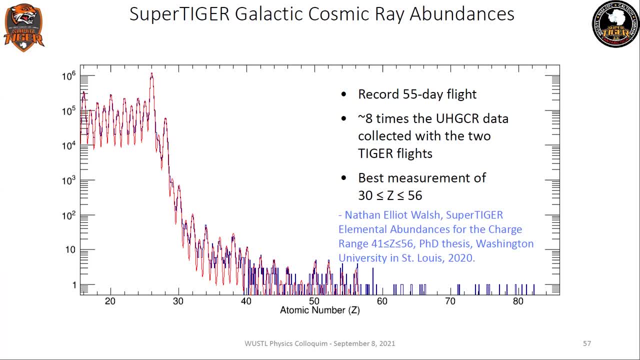 And we're still working on the scientific implications of that. But one other thing to point out here is: you can clearly see that we are out of statistics if we go any higher up, And we're also in the problem where it's very difficult to predict the charges, where 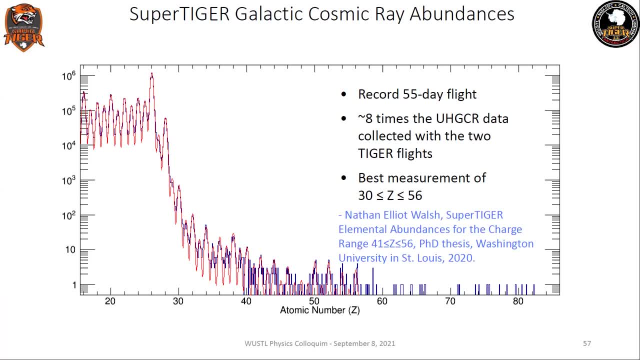 you don't have peaks, And with scintillators there's saturation effects that make it hard, So it would be really problematic to try to make measurements to higher charges with separate balloon flights with this instrument. So, OK, what did we get out of tiger? 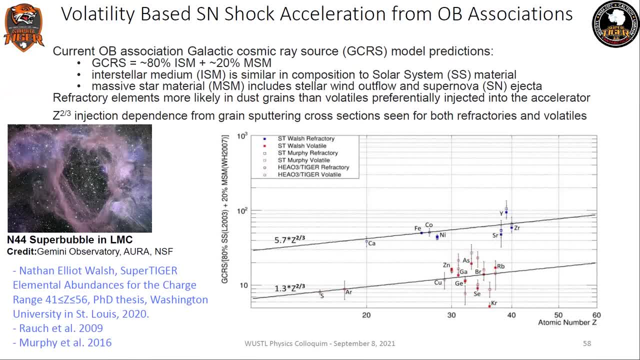 We got out of tiger and then confirmed this with SuperTiger results, a volatility-based supernibular shock acceleration model from OB associations. And this we had a lot. We got a lot of help from Kettering and Ladders. We suggested the nuclear composition. 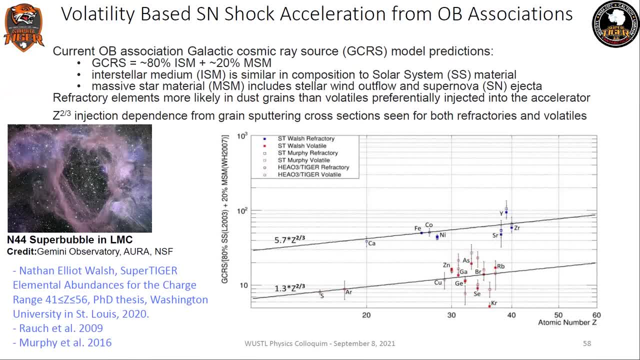 of material from massive stars, a special composition fraction, about 20% of the material that comes from the winds and outflows and the supernova events themselves, mixed in with something like 80%. regular ISM interstellar medium does a good job of ordering our data. 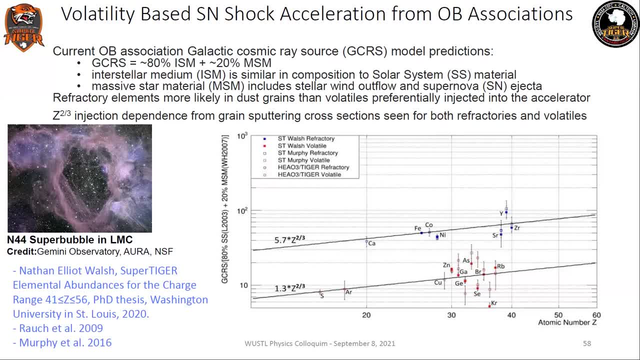 And our data. then, with that mixture model, pumped neatly into two lines, the top of which is for factory elements, those most likely to form dust grains that condense onto dust grains, And then the other, lower grouping, is volatile stuff that's less likely to 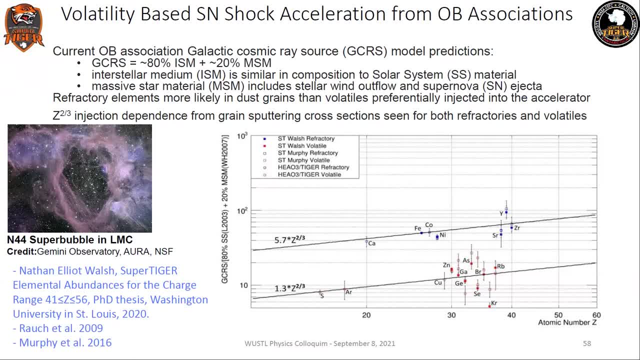 And then you have trend lines that go as approximately 0 to the 2 thirds. And this is expected because the model has that the shockwaves will accelerate the dust grains. Dust grains will have a small surface charge from photoionization, So they'll be very rigid particles, very little charge. 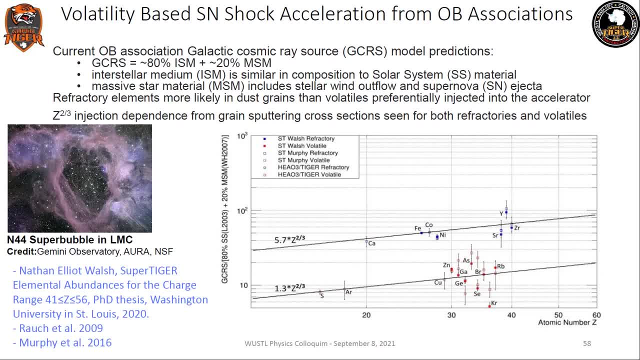 very high mass And they'll be accelerated super thermal energies. And then the atoms in the dust grain will get sputtered off by colliding with gas, And then they'll be preferentially injected into an acceleration mechanism that drives them up to almost the speed of light. 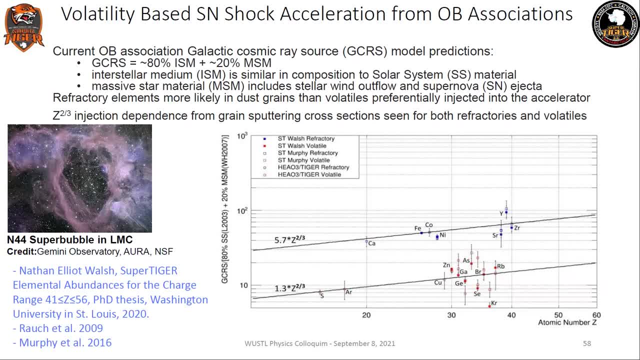 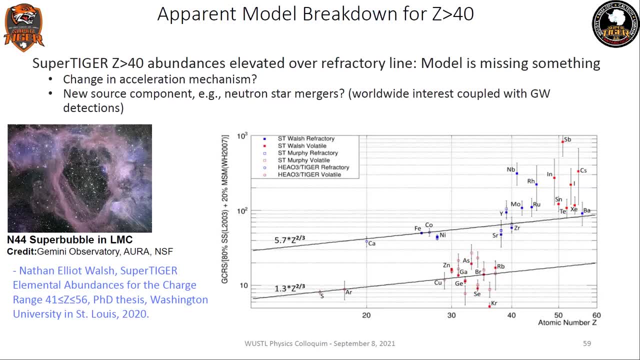 Well, you see, we have this nice, this model works. We've got good agreement, reasonably good agreement, And then we get Nathan's results pushing it out to 56. And, oh boy, We broke it. It doesn't work. 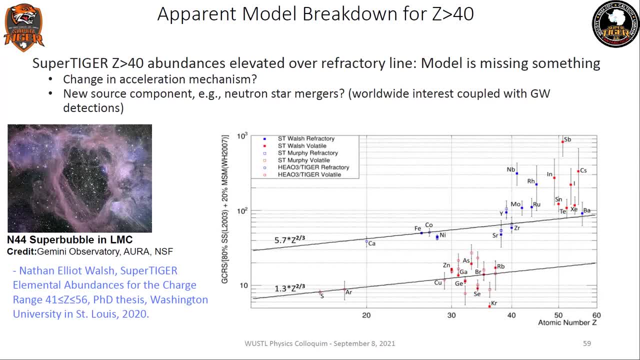 Something is totally different here. All the data are clustering above the refractory line. Not just the refractories, but the volatiles are all there, And it's a good question of what exactly is going on Now. the odd elements are the ones: 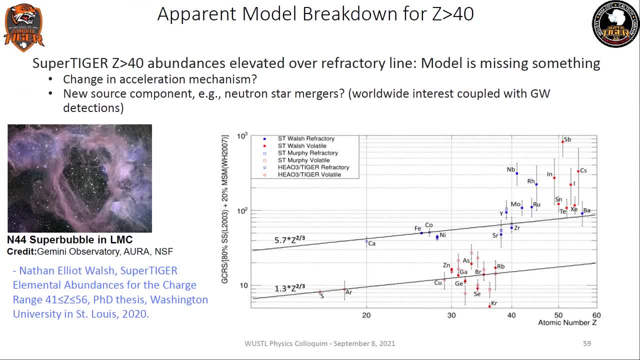 that are above with the bigger, much larger uncertainties, And so if you just look at the even ones, which are relatively more abundant, they're all much closer to staying together, But if we exclude the odds, we're still elevated above the refractory line in all cases. 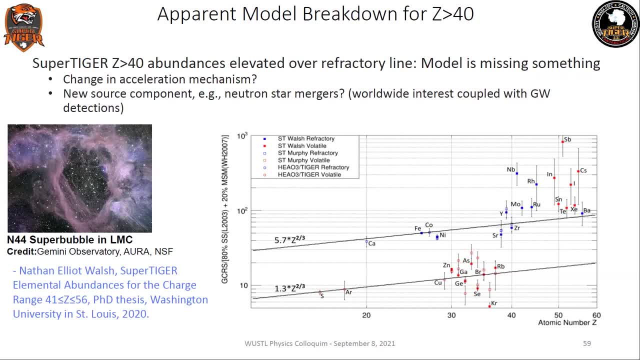 including volatiles. So that suggests that our model is missing something, And it could be that there's some different mixture components that we should be mixing in, Or it, I think, is more likely that there's something about the accelerator. that's. 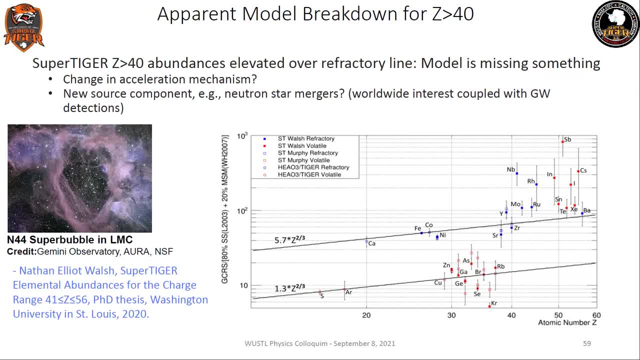 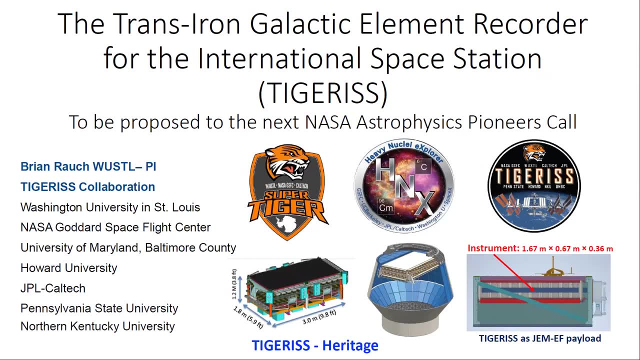 different for these elements. But in order to address such things, we will move on to the future. We hope to propose This next year, for the next NASA Astrophysics Pioneer is called the Trans-Iron Galactic Longer. Reporter for the International Space Station. 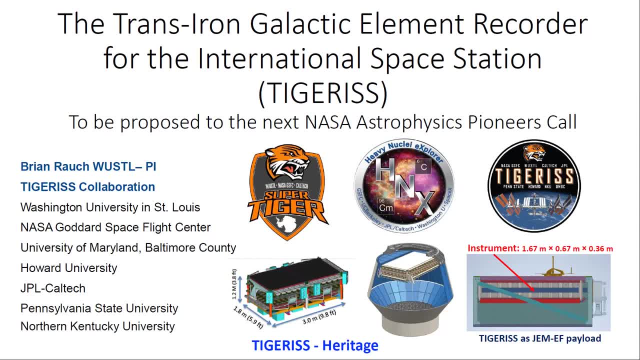 or TIGRIS, including many of the same groups that have been part of TIGR, but also adding Howard University, Penn State and Northern Kentucky University to the mix of folks, And, of course, this builds on SuperTIGR. 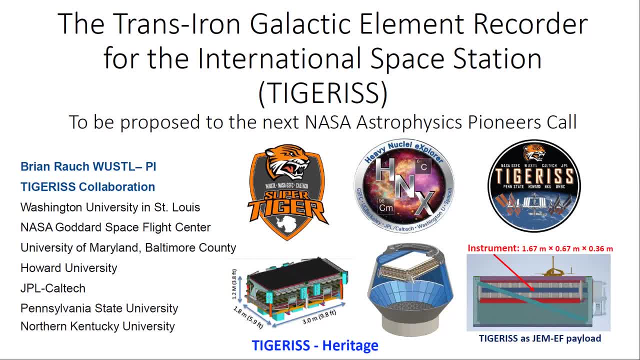 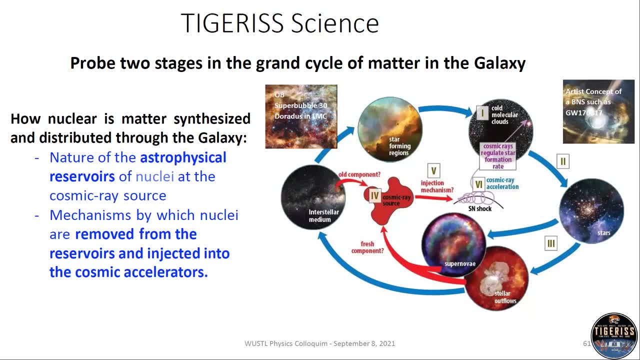 and in a previous heavy nuclear explorer proposal that we put in that didn't get selected but was well reviewed, And just pulling a pretty picture from that proposal. this is the material. We've aimed to probe two stages in the grand cycle of matter. 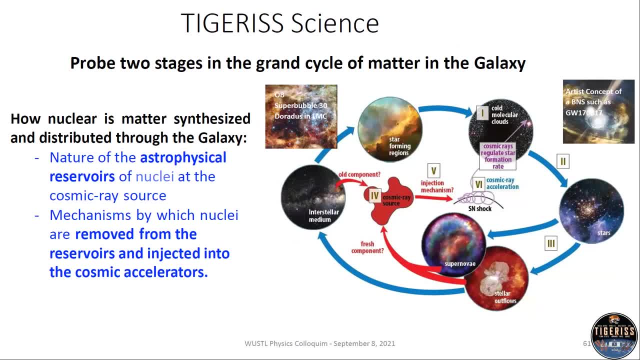 in the galaxy, And you've got to use these big words and proposals right. Cyanonuclear matter is synthesized and then distributed through the galaxy. So what's the nature of the astrophysical reservoirs of nuclei at the cosmic-ray source? 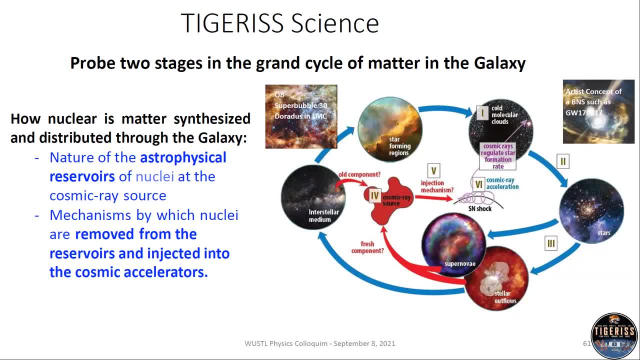 Well, we thought that it was OB associations That explained everything, but maybe there's more to it, right. That's why we need to probe higher and confirm the SuperTIGR measurements. Also, mechanisms like which are removed from the reservoirs. 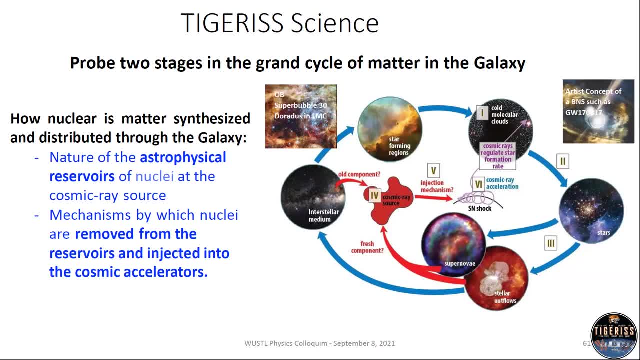 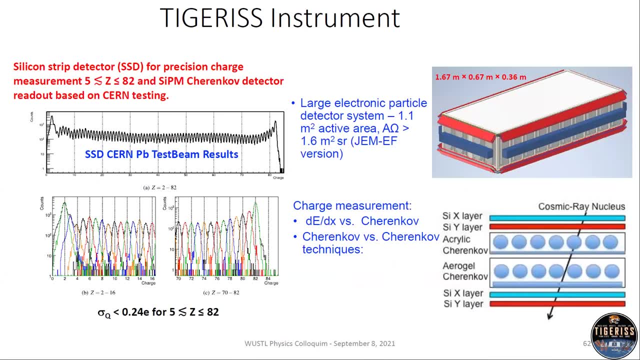 and ejected into the cosmic-ray accelerators. Well, we had a nice model, But that's no longer quite working, So there's real incentive to keep pushing on this. So the TIGRs instrument shares many of the same characteristics of the SuperTIGR type of instrument. 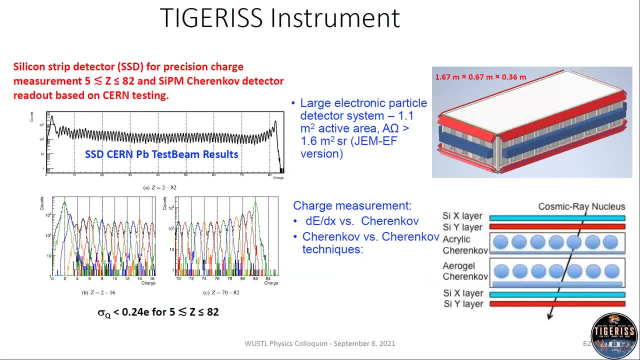 only it has silicon layers instead of simulators, which have far better, more reliable charge response as a function of charge. It's much easier to make a measurement and you think it's a lead? 82. It's far more likely to build. 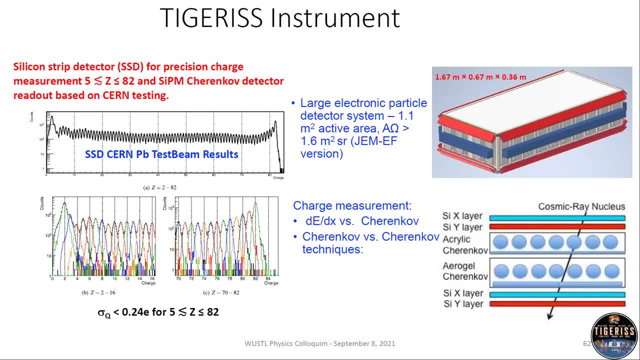 Lead 82 than it is to be misidentified when you're using silicon. It's just better resolution. It doesn't have saturation effects. that are a major issue And the curve showing the solid-state detector, silicon strip detector there is from a certain lead beam test. 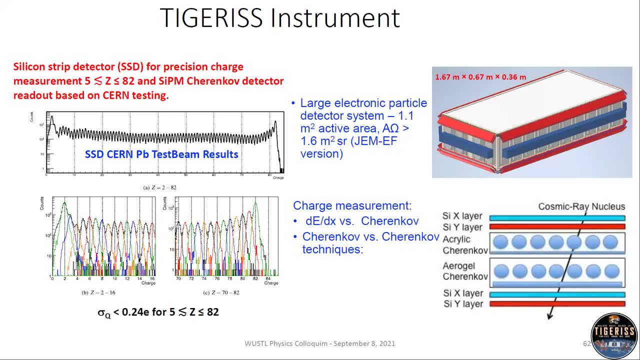 where you see the fragments. You see lead peak at the far right and the fragments all the way down And the peaks are identified. So it would still use Trankov detectors, acrylic and aerogel. So it's very similar And this is a TIGR. 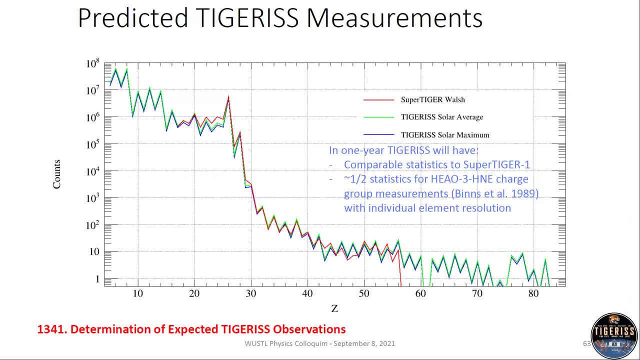 This is what we would predict for one year from TIGR on the space station And that's the basis you have to propose for with astrophysics pioneers. You have to get your science out in one year. And I show the predictions for solar average and solar maximum. 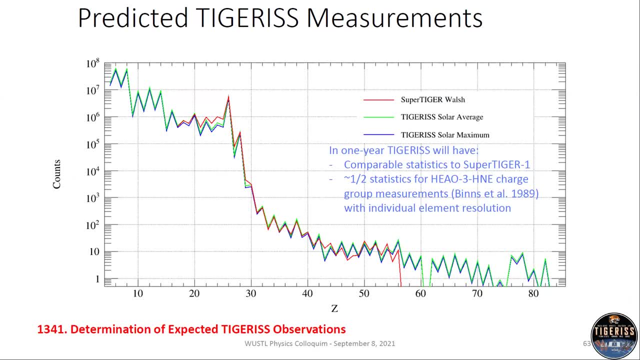 And solar maximum is the worst case scenario. But you can see there's very little difference between the green and blue lines, which is an effect of being within a geomagnetic field. The low energy stuff's already screened out And the solar field would screen out the rest. 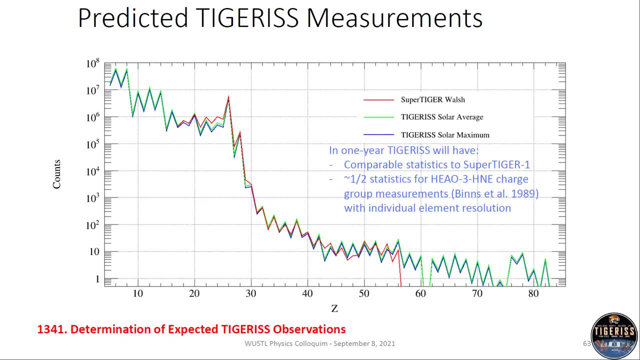 The red line is the super TIGR measurements of Nathan's And you can see that basically we would get similar statistics to Nathan's super TIGR all the way through barium, But we would also have some preliminary resolvable measurements out all the way to lead, lead flattening. 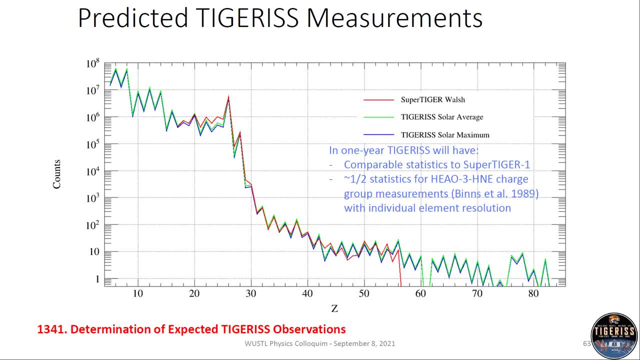 And also I think I have about half the statistics of that HEO hyponucleic explorer measurement that I mentioned earlier as the existing best for above barium, And you can see there's a lot of data, So we'd be able to check that and also begin. 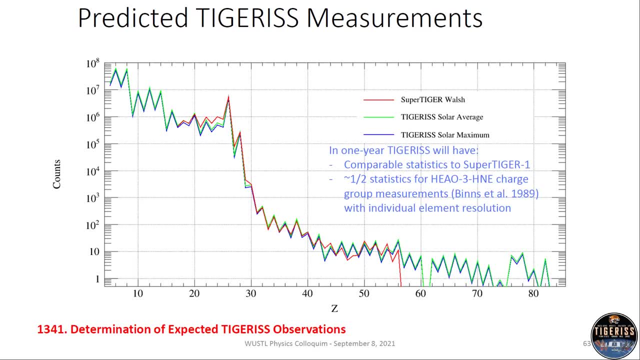 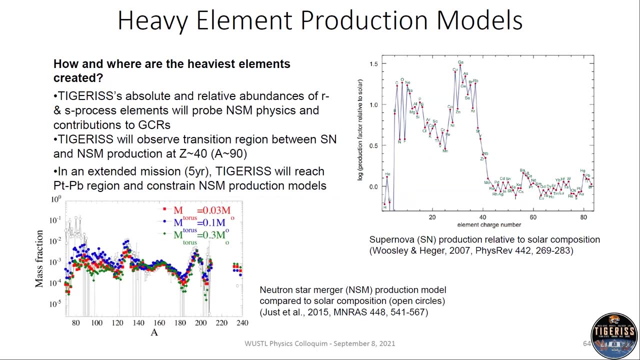 to see how the events are falling in large charge groups that they were able to resolve, And so, again, the main focus is to try to understand what the source material is and the accelerator injection. And the figure in the upper right is what we get from supernova production and massive star. 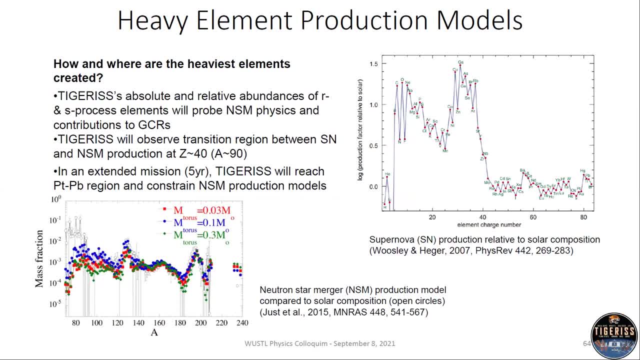 outflows, And this is what Kettering and Lauder put us on to way back when we were doing TIGR. But now that we know that it's been seen that binary interest for mergers do eject matter, That matter is seen to be composed of heavy nuclei. 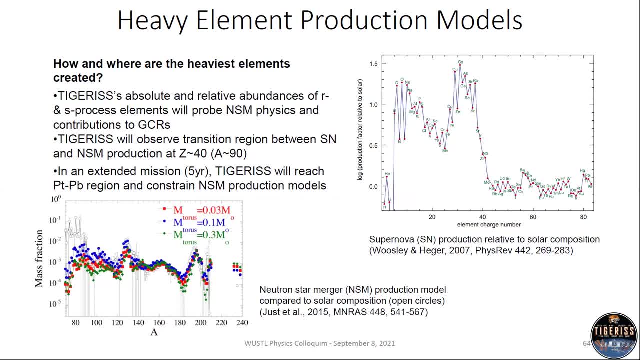 That's a definite source of the heavy IR process, And so there are models in the bottom, for instance the bottom left, showing what you might get out of merger type events, And so, by probing the abundances of elements further up the periodic table, we 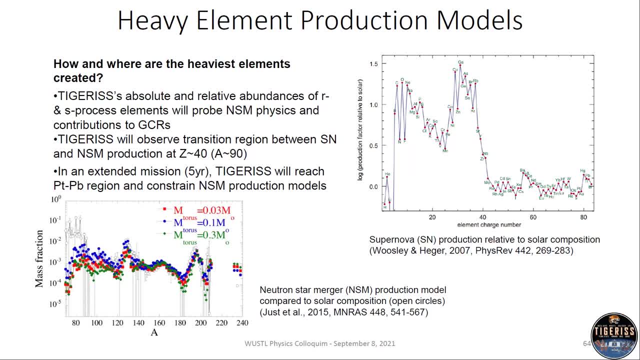 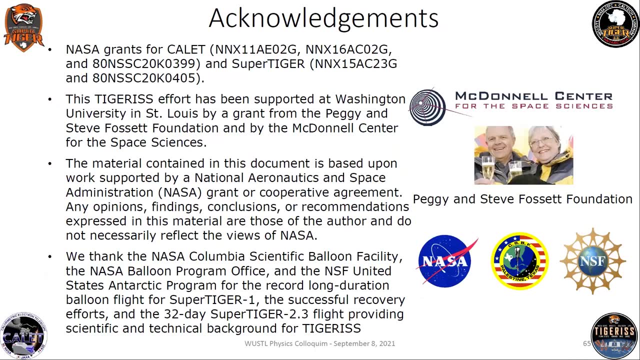 can hope to determine what the relative contributions might be to not just the cosmic rays, but also possibly also the sources in general for the heavier elements. And this is just the official acknowledgments Thanking NASA for funding both KEL-ET and SuperTIGER. 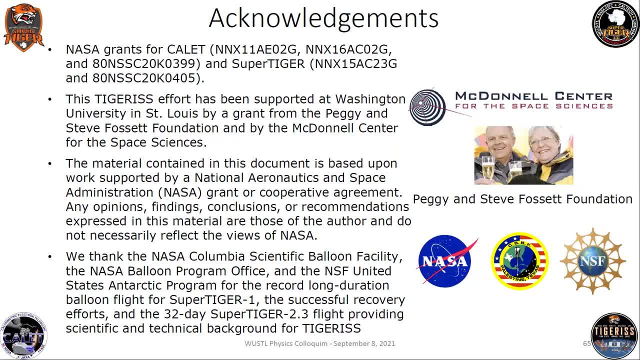 And TIGRIS has been already gotten support from the Center for Space Sciences and the Peggy and Steve Fossil Foundation. And then we have the standard disclaimer, because this is grant supported in some way, but NASA's not responsible for all our mistakes. 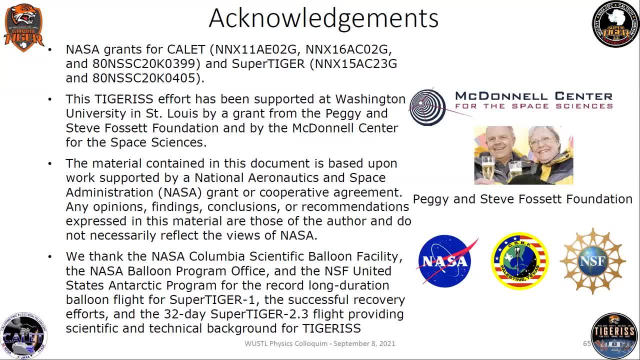 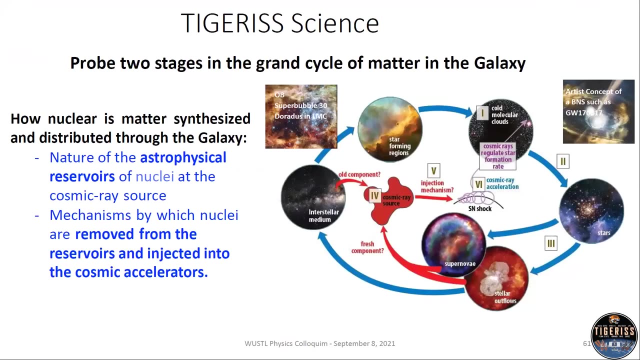 And that would be it. Thank you, It's 10 minutes. That's not the worst amount of time for questions, if there are any. Brian, a couple slides back, maybe on your advertising slide you had a treating statement. Cosmic rays: regulate star formation rate. 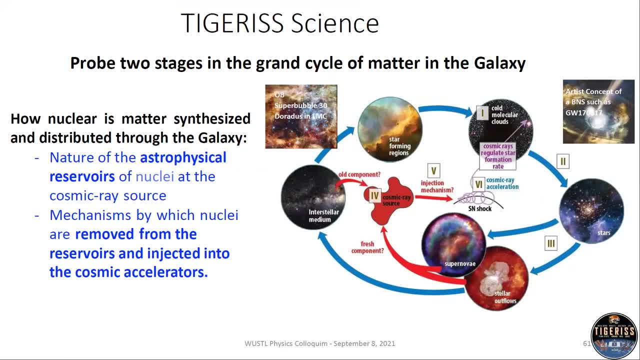 What do you mean by that? OK, well, they feed back, So they feed into the magnetic fields And By supporting and partly supporting magnetic fields, that kind of counters, It's like it's a pressure that counters star formation. So the degree to which they're driving magnetic field, 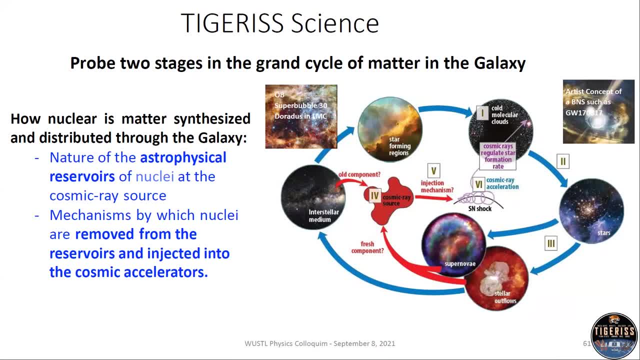 impacts that. I think the exact details are beyond me at the moment. I just have to know them better for that part of the proposal. I didn't make this particular thing. You might just say how the energy density in cosmic rays compares to magnetic energy density in starlight. 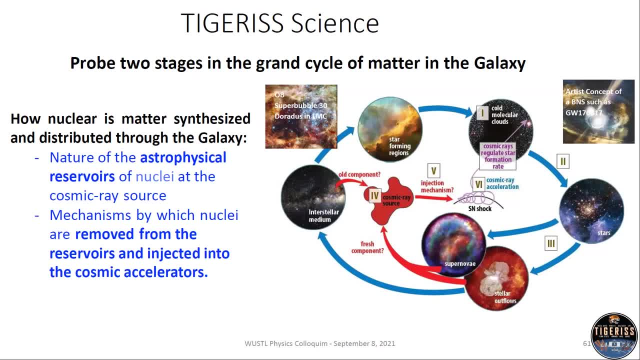 Yeah, right. Well, I mean basically they're equal partitions, As I remember from class, about a third of similar power budget in starlight, magnetic fields and cosmic rays. Yes, Yeah. so when you showed the plot of the calc data you showed. 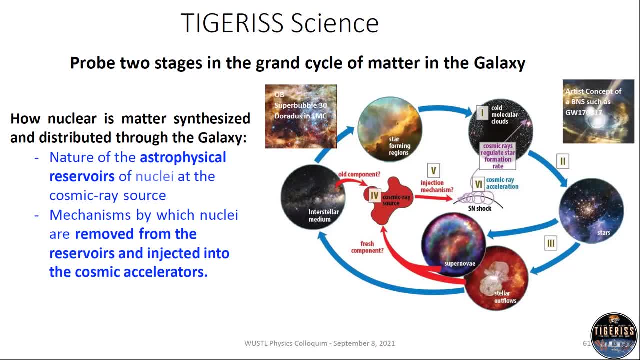 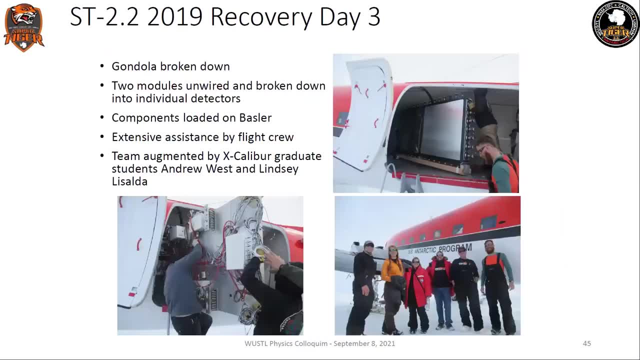 how, like, the different experiments disagree. Can you maybe tell us just a little bit more about? are there certain systematic errors that you might be concerned about when comparing different data sets? So you're driving all these sides, So all right, So all. 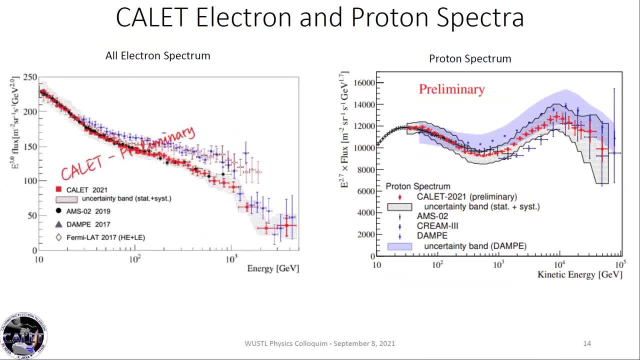 So yeah, these kinds of plots, All these are space measurements And but they're not the same type of instrument, right? So there are magnetic spectrometers, like the alpha magnetic spectrometer on the space station, where you have a magnet, so you can really 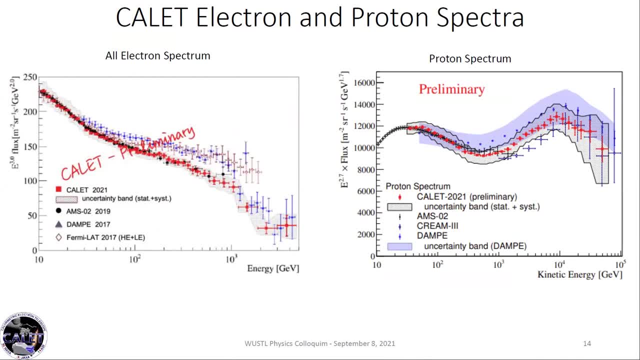 to help determine energy, And that's a more reliable measurement of energy, as a rule, in principle, than a calorimeter, Because calorimeter the energy deposition is complicated by, especially if you talk about nuclei, If it's an electromagnetic shower. 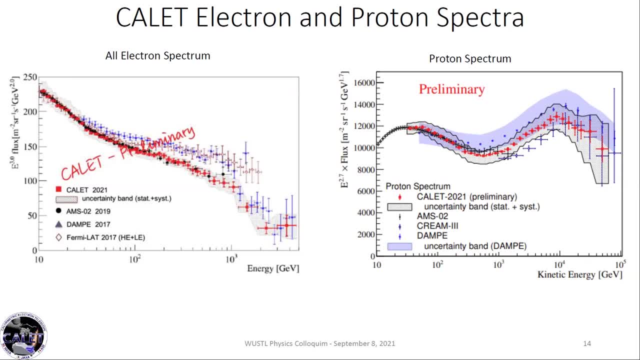 if it's just an electron or a photon showering, it's much better. It's easier to predict the calorimeter's response, But with nuclei the fragmentation cross sections aren't as well known. So that's why we go with accelerators. 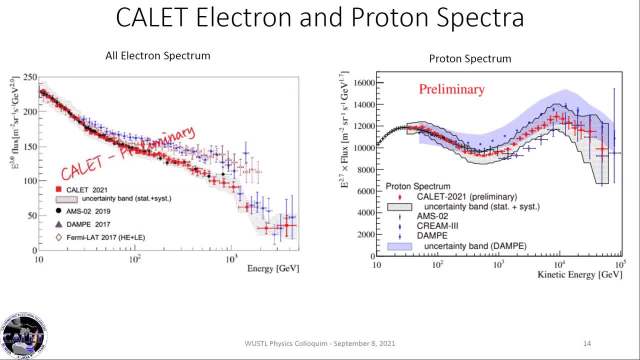 and we use multiples. So that's why, in fact, we use the three simulations to try to get a handle on what the systematic uncertainties are, just from that deconvolution of energy based on the simulations, Because we have to use Monte Carlo information. 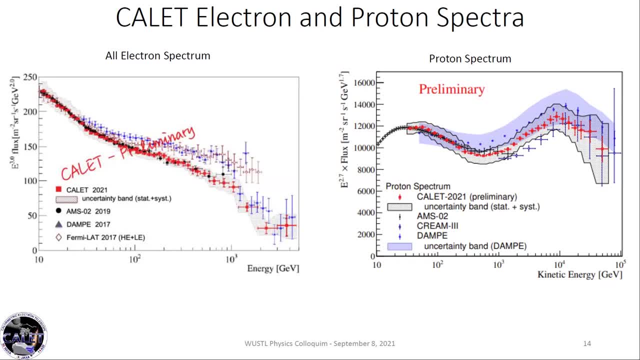 to tell us what instrument response, what that instrument, what energy corresponds to that. So there are those features that are certainly part of our cal-let uncertainty. And then the crazy thing, of course, is the calorimeters don't agree in all cases. 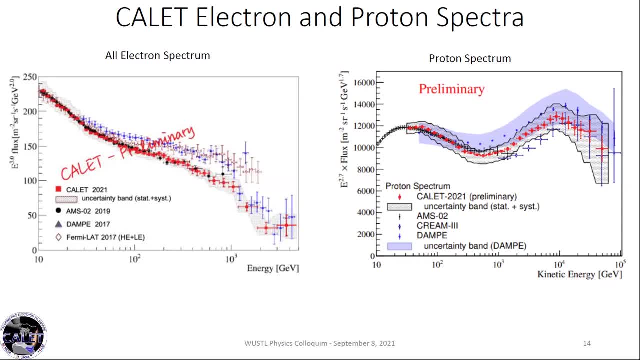 If it were like the calorimeters, magnet spectrometers were always two separate camps, They'd be one thing, but they're not. Sometimes one magnet spectrometer agrees with the calorimeter and other times the other one does It's. 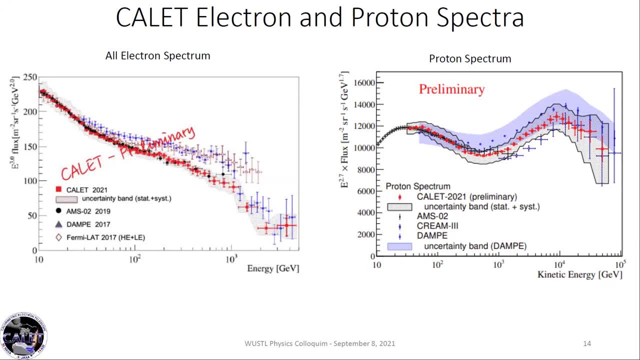 There's also Dampy, a Chinese free flyer that's similar to cal-let in capability, slightly larger. That's on the end. It's indeed plot ends. You see Dampy data points And they're contemporaneous. We met them at CERN doing their calibrations. 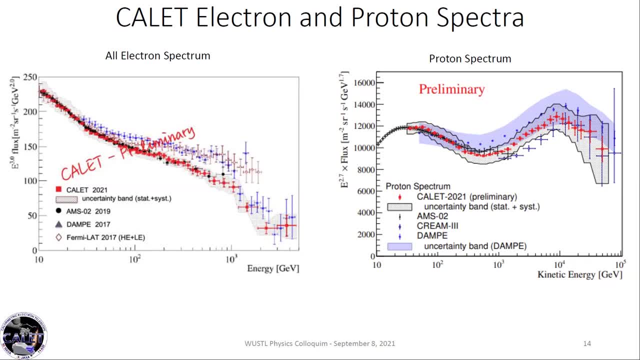 And again, sometimes they agree with us and sometimes they don't, And they're another calorimeter instrument. So it's just one of those mysteries where a lot of it comes down to which simulation you're using, how you're using it. 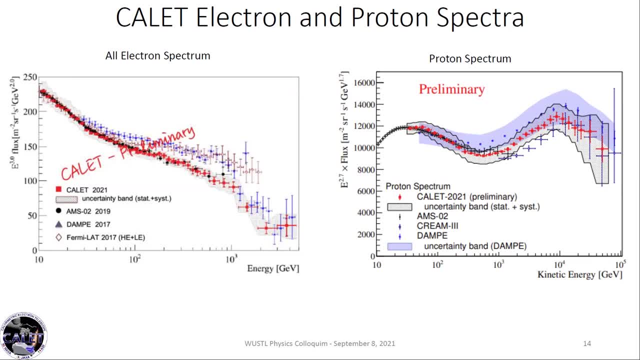 And cal-let's been looking into not just the simulations used by other groups but the exact configuration. So we've been trying to do simulations using the same version of Jayant, that say, AMS is using the exact same version like configured the same way. 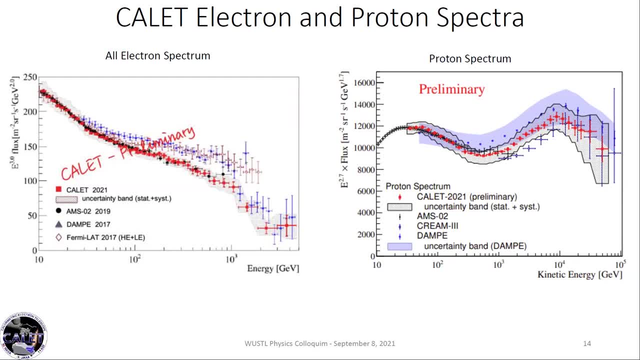 And so far that has not been the magic bullet that explains differences, But it does definitely show differences, And so the problem is, you do have to rely on the Monte Carlo and the modeling, And that has its limitations. So that's why it's best that we have local instruments. 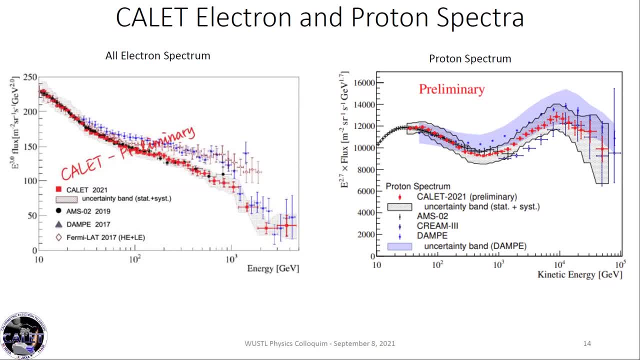 I think what's next? Buckley, Oh Buckley, Oh well. sorry, Jim, I'm used to you speaking up. Yeah, no, I was trying to be polite, uncharacteristically, So I was just saying, All right. 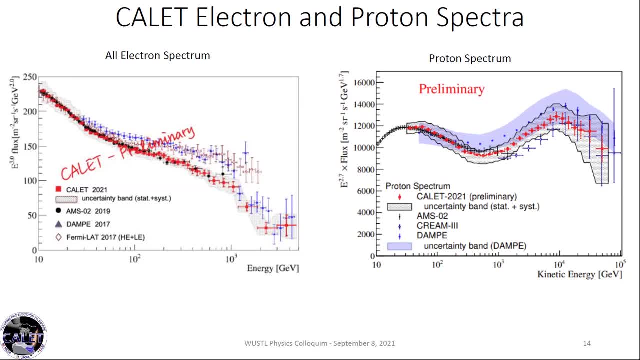 I was just going to say another WashU experiment. Veritas measured the spectrum out to higher energies, in degrees, I think, with the upper curve And before that Hess in an independent analysis saw it. So these are ground-based gamma-ray instruments. 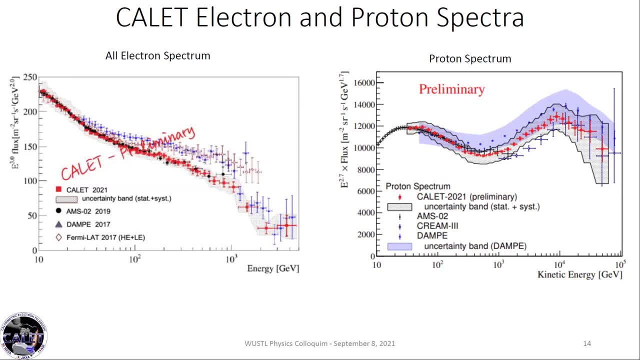 They have a huge effective area. But the systematics for this type of study are viewed to be worse than these direct measurements, which is probably why one might choose not to include them. But they do kind of go a bit higher And energy. 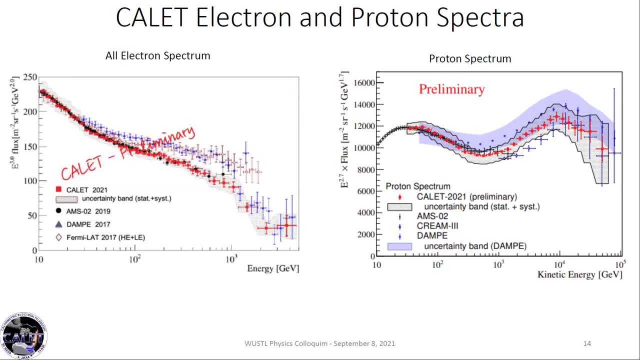 Yeah, Well, I know that in the paper those will be there, right? This is just the preliminary at the conference one, And I just put these because they're the most recent. And yes, of course, And that's the exciting thing, though, is here's an instance. 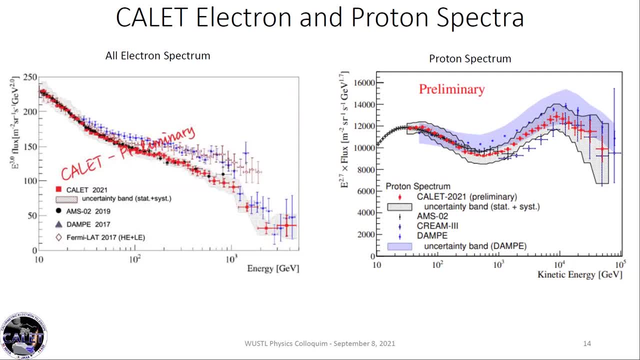 where you're getting overlap in measurement between direct measurement in a regular size detector and a ground array that's looking up at the sky Right. So that's an interesting region of cross-correlation, And the total electron spectrum and of course the positron fraction are of great interest. 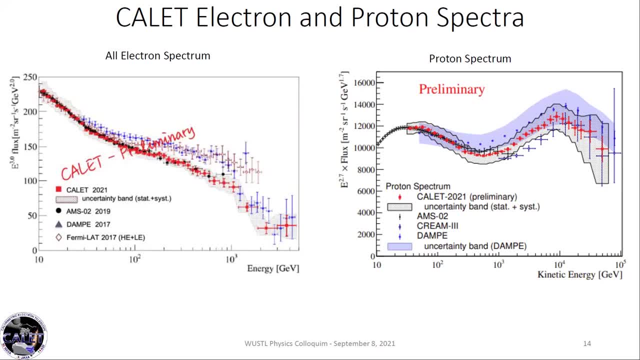 to things like indirect dark matter detection and other more exotic things that could contribute, or nearby pulsars and so on that could contribute. So it's a good thing to look at. Yeah, And I neglected to mention that Kellett measures the whole electron. 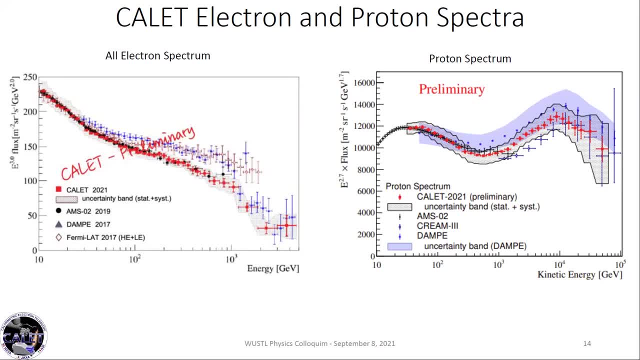 spectrum because they can't distinguish positrons from electrons, unlike EMS which has the magnet, and they bend the particles And endoparticles, And endoparticles bend oppositely. At Jim's suggestion we did look at the range of which we could use the geomagnetic field. 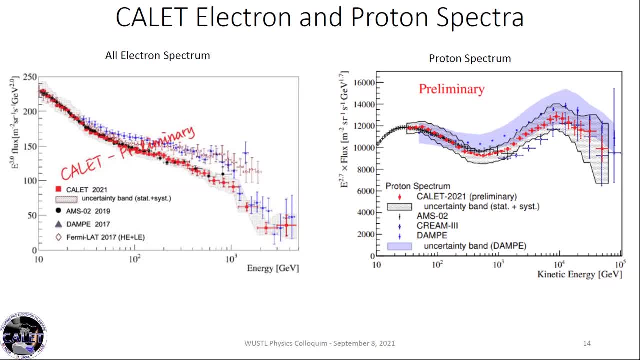 to distinguish electrons and positrons And there is a limited energy range- And I remember off the top of my head because it's been a long time since I wrote that paper- But it's a limited range, But it would be a measurement. 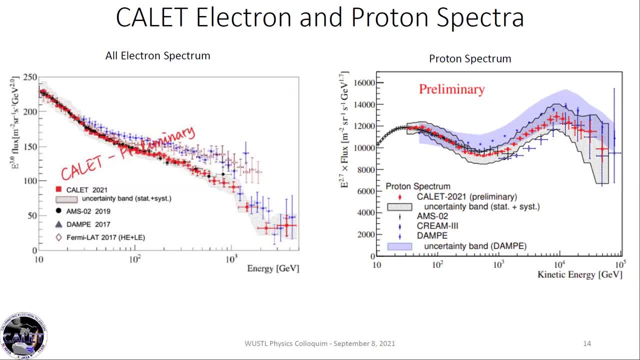 And it's the kind of thing you could make a grad student do if you had one that had any free time. So I guess I'll add to Manal: Sorry, So you showed that for the proposal where you're applying to put a sort of tiger-inspired instrument. 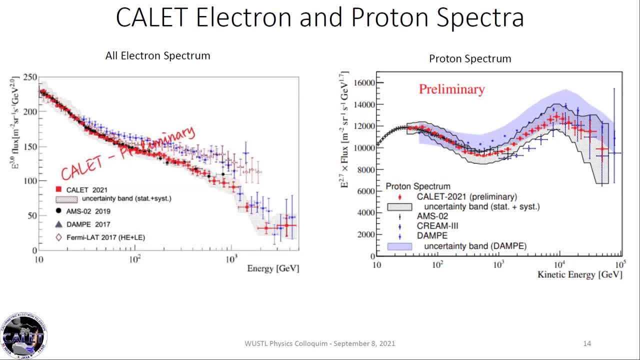 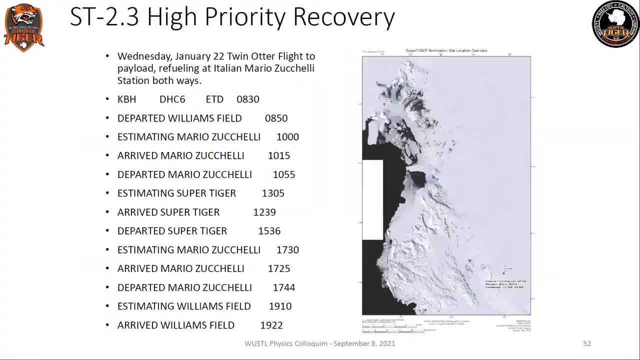 on the ISS. Right, You showed that the expectation was that the statistics would be similar to the data from supertigers that you already have. So is that just a matter of size, or the one that goes in the ISS has to be smaller? 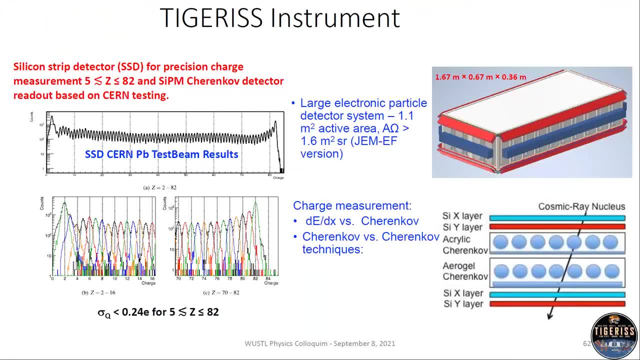 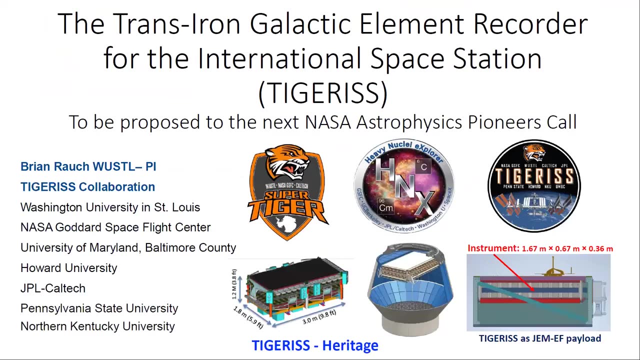 Or is it that you optimized this one for the heavier element? It is the comparable statistics in one year is a function of relative instrument size And we like that bigger. But we are constrained to fit in the box And the box is a refrigerator-sized box. 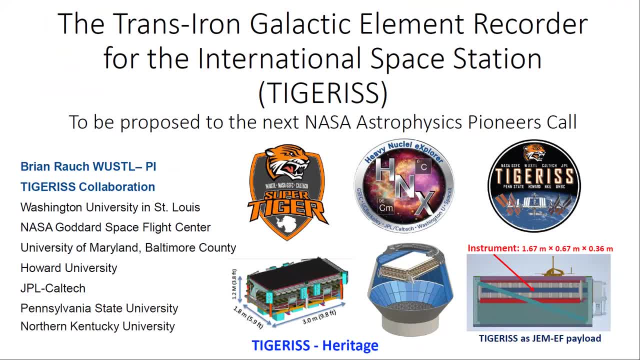 And supertiger had those two big modules And also supertiger. so flying by holes at least you don't have the geometric screening in any significant way. But then the atmosphere does a really great job of screening too, And so the energy ranges for supertiger and tigress. 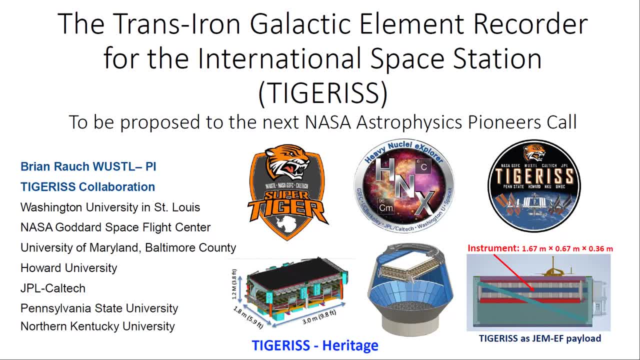 would be rather similar the end, Although it'd be really nice not to have to do atmospheric corrections, which is the part that I do for SuperTiger and Tiger, and don't trust the person doing it so much so I'd really like another space measurement which reminds me of again the real value in 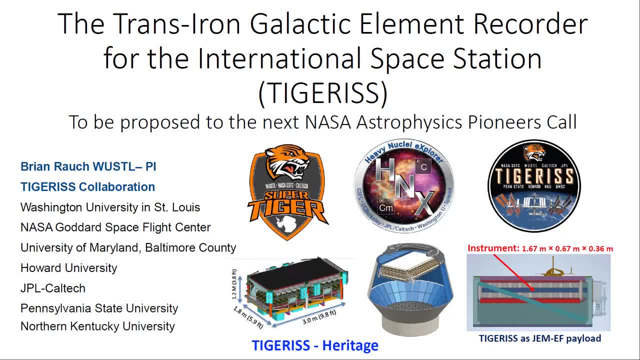 Wolfgang's cal light measurement is not just that it's a significant measurement in its own right, but that it also is a comparison with totally different systematics where we have geometric screening to worry about. but that's much easier. I think that's really much easier to get a handle on than the atmospheric corrections where the cross sections are so 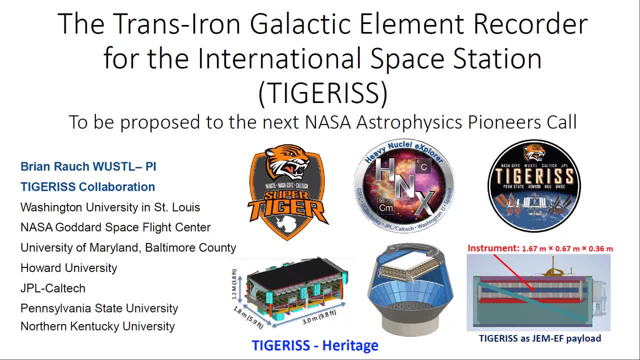 uncertain and you have to make very gross assumptions to correct. for I can't do fine degree, I can't do fine corrections for like bins of incidence, angle or energy or anything, because you know the ultra heavy statistics are so low. I just have to do one global correction. 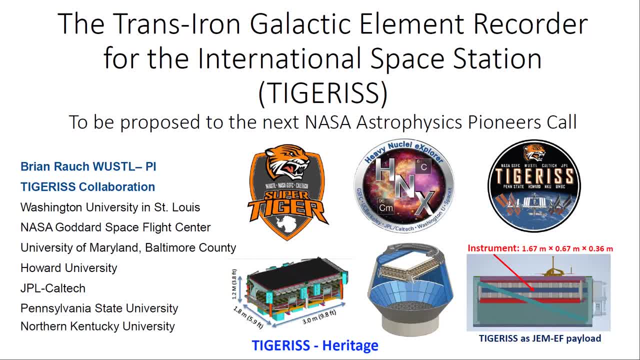 and then assume, have an analysis. So it's an average atmospheric depth and that's fishy, so it's. it's been encouraging so far that the cal, lat and indeed ace chris measurements have agreed as well as they have with what we've shown previously in the Tiger and SuperTiger. but that was a side sorry. 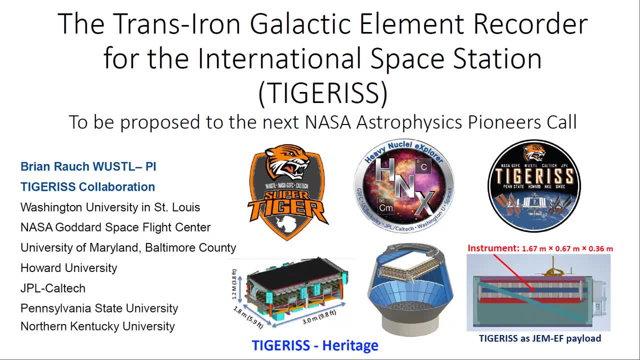 Mike. A few more questions on on the calibration. So, since you get to pick up your instrument after you're done with it, with SuperTiger, yeah, yeah, do you, at least sometimes, hopefully, do you? Do you do pre-flight and post-flight calibration, or just to see if it changed? 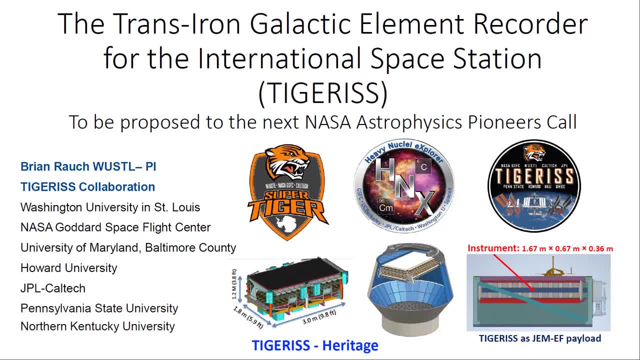 You know, I'm looking from the perspective of satellite, where the agreement between the different instruments is excellent as far as anyone is concerned who flies the satellite, because they never agree to better than, like you know, 10 or 20 percent. and I guess the the second question related to that is for the simulation tools. they're going to be a 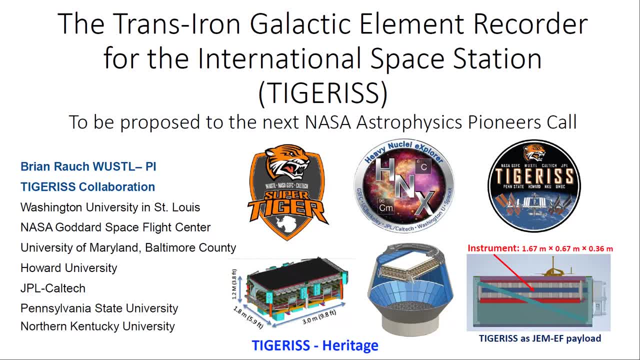 combination of theoretical modeling and data input, like cross sections. you know, I feel, what the differences between the different simulation tools are, in terms of whether it's closely related to the theoretical modeling or the database input into the models. So, all right, I guess I'll start with the second question. you have to remember the first one. 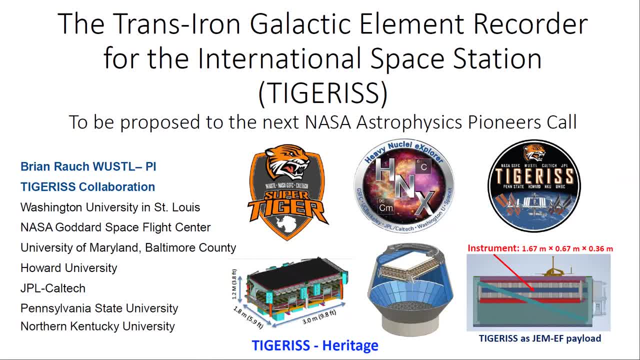 again when I get back to it. but, um, you can usually pick um this. you know, like the cross-section physics models, you can choose to be the same between simulations and yet they still have their own differences, of course. Yeah And um, the epic simulation that is the primary for Kellett because one of her collaborators 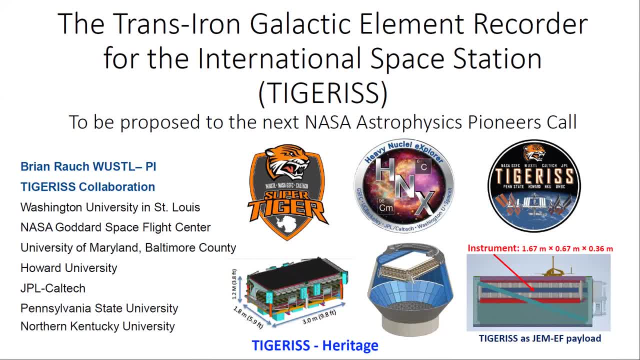 was the original author of it. um, you know, I know that, as throughout both the, the beam test phase and the actual data from on flight, you know they've been checking and checking and finding things that are quite right or missing or or where the the simulation crashes. 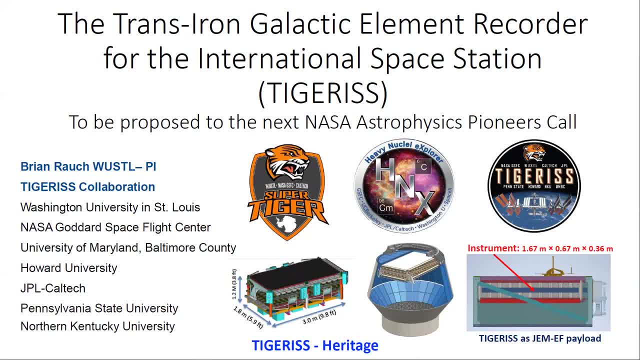 because it's overloaded um. So there's- Yeah, There's- a lot of nuance, a lot of differences between the packages and and finding them is not not easy. I mean one particular area um where there's can be significant difference is um backsplash. how much backsplash you get from an event in you know that's really important. 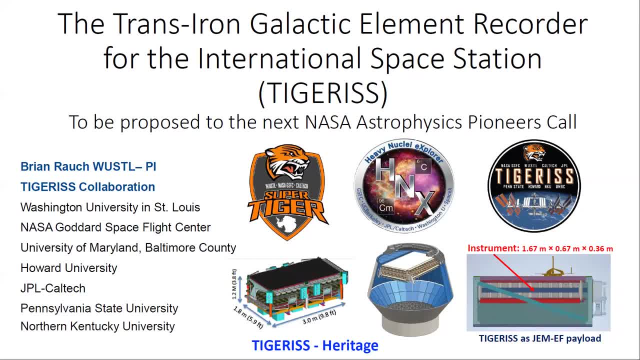 in calorimeter you have all this dense materials because you're trying to capture the energy, but when you get interactions and you're fragmenting, stuff will bounce back, and being able to properly model that there's been some real differences between the packages there. Yeah, 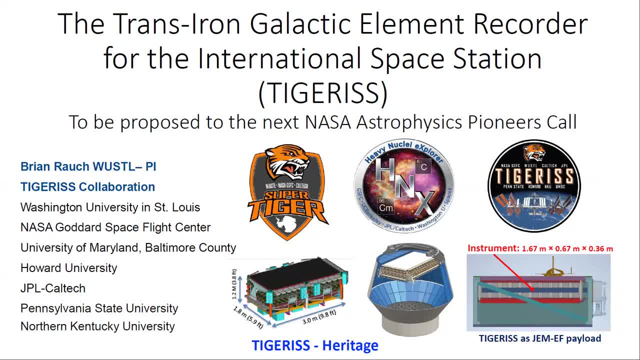 And I don't know the degree to which that would be a function of the basic physics models. I don't think it would be that strong, but clearly there's some difference between the packages, that you're seeing, a difference in the backsplash. And then, um, do we, you know, calibrate? well, the super tiger? we, we don't. generally, we have 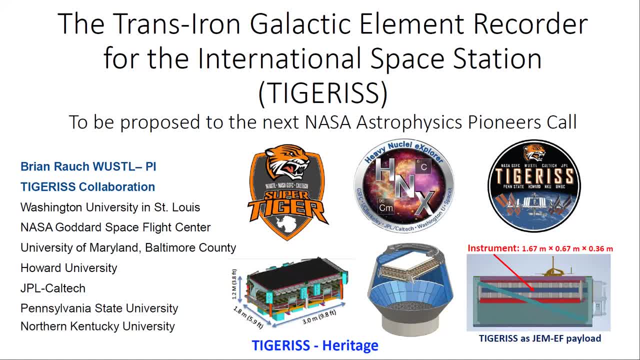 taken super tiger detectors to accelerators for for trying to calibrate the responses and understand the simulator saturation effects that make it hard to predict charges, the higher at the periodic table, um, but we haven't made a point of doing like a full instrument beam test, kind of cross calibration. um, we, you know, obviously you know, we put it back together on the ice and we. 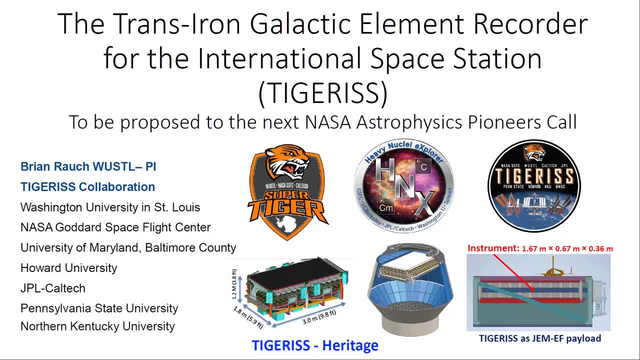 were doing tests, many like the tests, the cross calibrations- we were able to significant, most significant ones are muons, right, so we we did look at the muons. um, we had muons runs from before we flew and crashed and reassembled and after 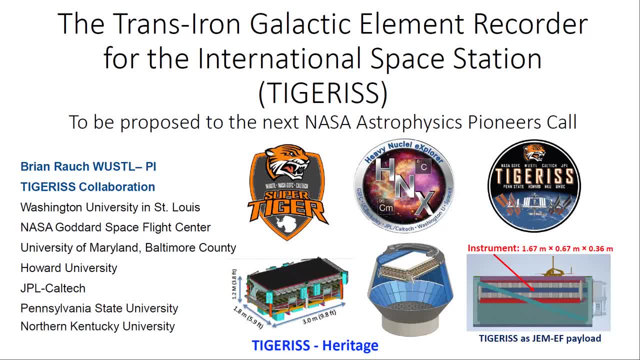 And they were. generally they were. they were acceptable agreement, I guess, is the most I can say at the top of my head. Um, but yeah, we probably don't do as much in that way as maybe we should. But yeah, after we get things that are kind of busted up, and it's, it's the state, it's in. 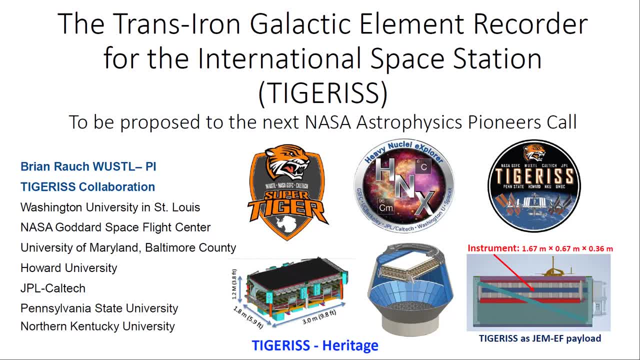 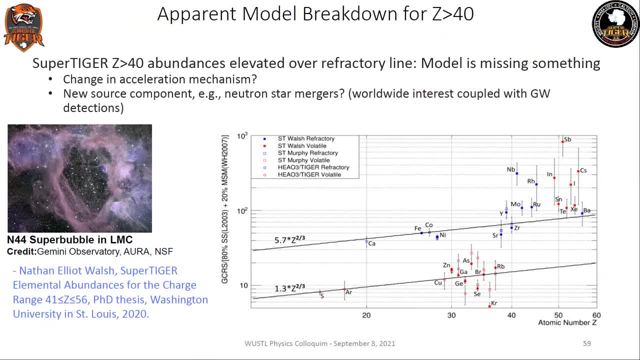 And Henrik The super tiger points were well above the line. but so do you think it's made a discovery or does someone have a discussion? This, oh I just the model's missing something. um, I, I have a pet theory about it's an injection of accelerator, but I, yeah, there's, there's something here. um, I don't think it's going to be a science paper by the time we're done with it, but it certainly is interesting and hopefully is enough to build interest for for another instrument. 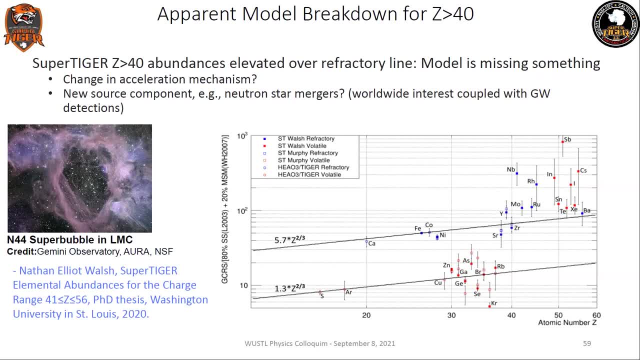 How does a FIP model look at first ionization potential? Well, when we looked at it, it doesn't agree anywhere, as well as the volatility. but I guess we haven't, Nathan, we have not looked to see if somehow that FIP is magically working so much better for this group, that would be. that would be worth worth worth of being. and Nathan's nodding, so I guess we'll do that. probably not. yeah, there's that too right, I mean. and this whole model. 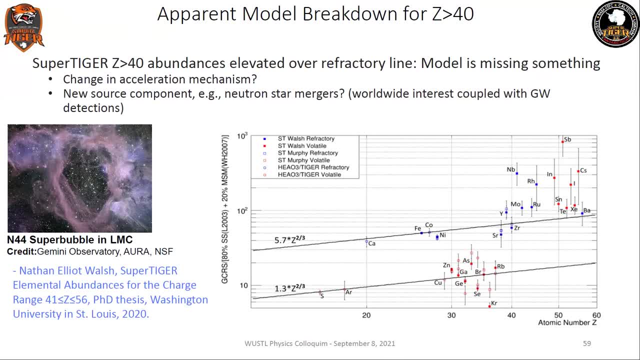 Is based on on, you know, grains. I mean, is it, are you accelerating normal gas? Well, so the assumption, so the original model seems that the grains and gas were accelerated differently, and it had it posited that the gas should have a mass dependence trend, but not the- uh, the grains, because it's the mass of the atom itself that governs its efficiency and acceleration, it's a rigidity of that atom. 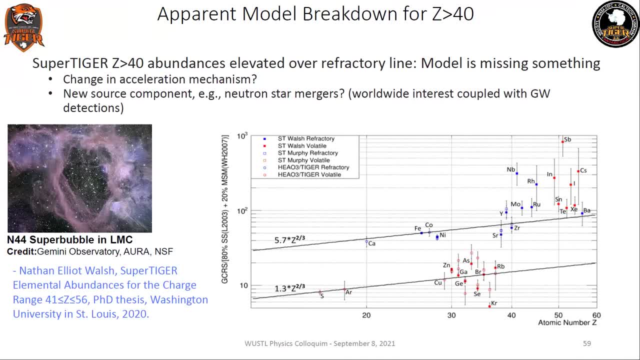 But here we found that you see trends for both the refractory and the bottles, and that that's where the sputtering idea comes in. it's the sputtering cross section that relates. the thought for why you would have a volatile in working in this model is that everything might condense to some degree on these grains, and so the bottles are just much less like even- but I mean even- the xenon. well, I guess, if it's cold or yeah, that's a great question. this is one of these things where 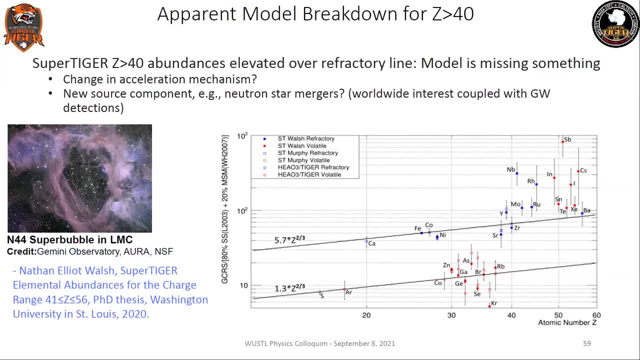 Where it's time for us to go talk to Katerina again To hear about that. Yes, I don't know if you can see me. I don't know what is going on. I actually saw this data for the first time right now, and my first. 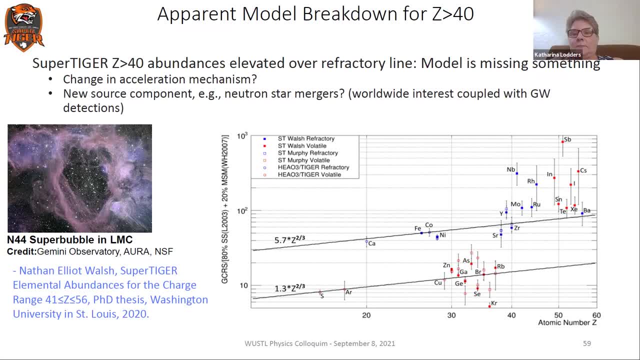 thought is that the barium peak region looks quite interesting and I wonder if that could be just a signature of the our process peak and since we still don't know how many different our process sites we have, I suspect that is a nuclear synthesis effect because of fractionation between xenon and krypton, rubidium and strontium, and also tellurium and selenium. strikes me as odd because chemical fractionation wouldn't work the same way. 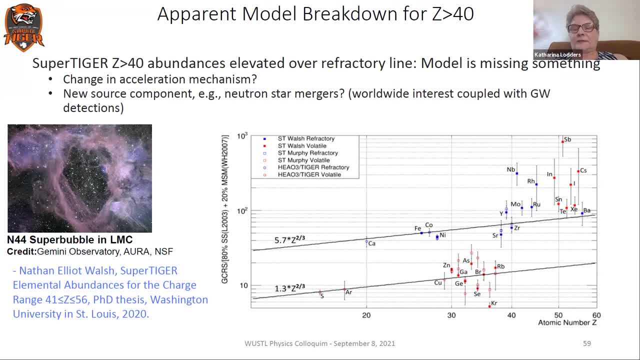 because chemical fractionation wouldn't work the same way, So it must be a nuclear effect. but this is just my first impression. I have to digest this data just as well. in fairness to Nathan, that was his first thought to. that was looking like in our process. yes, enhancement, and yes, that would be. that would, in a lot of ways, be the more interesting. 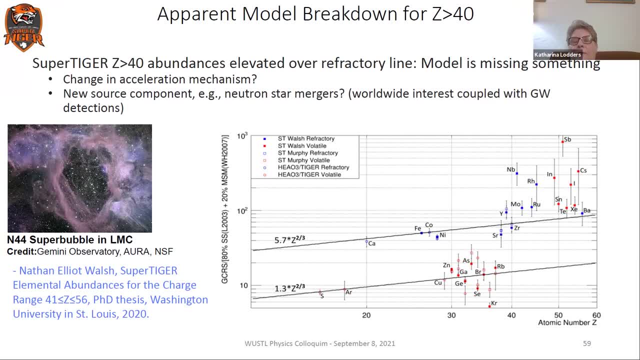 The other thing is I, the niobium is a little bit odd. so, and molybdenum stuff? I don't know how a P process would work, but it clearly needs to be scrutinized for nuclear synthesis effects. Well, thank you, yes. 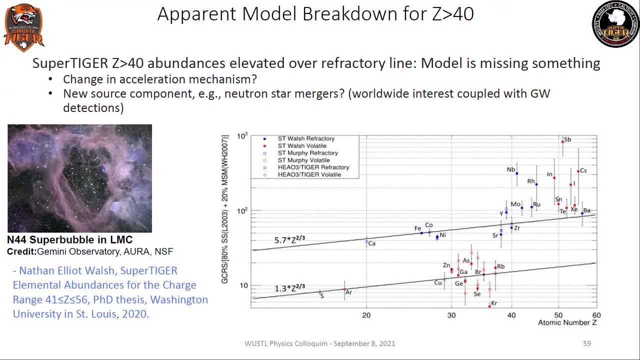 Okay, Thank you, Brian, Really interesting Again.